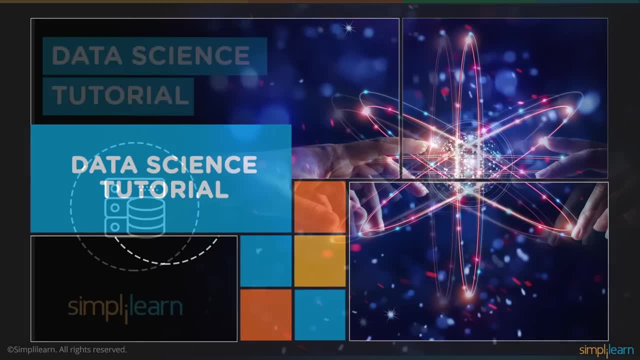 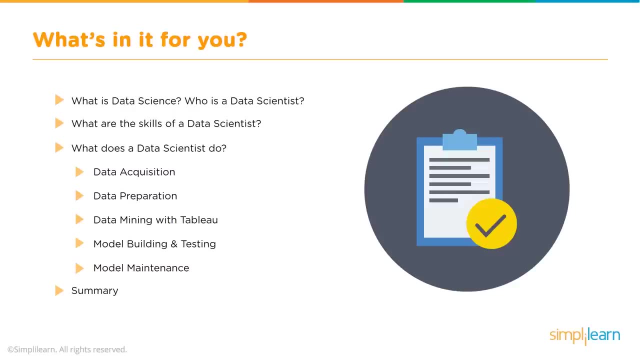 hello and welcome to the tutorial on data science. in this tutorial we are going to see what is data science and who is a data scientist. what are the skills of a data scientist and what does the data scientist do a day in the life of a data scientist? what is a methodology used for? 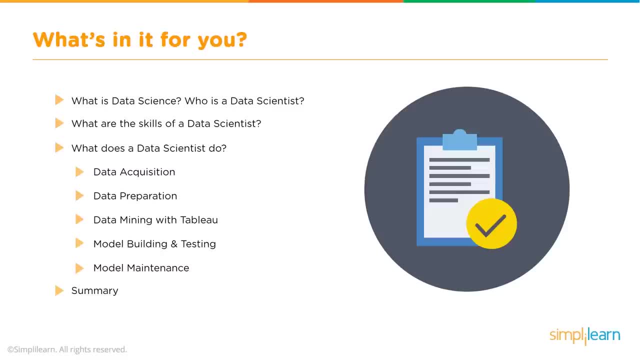 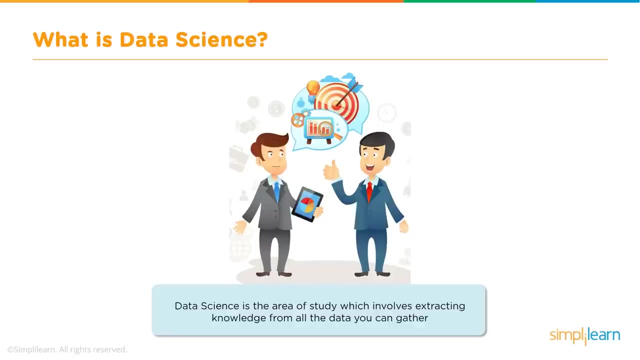 data science like data acquisition, preparation, mining and model building and testing and then maintenance, and then towards the end, we will also see an example program as well. I'll take you through a quick code where we have done some data science activity and then we will conclude. so let's get started. so what is data science? as the name suggests, it is nothing but study. 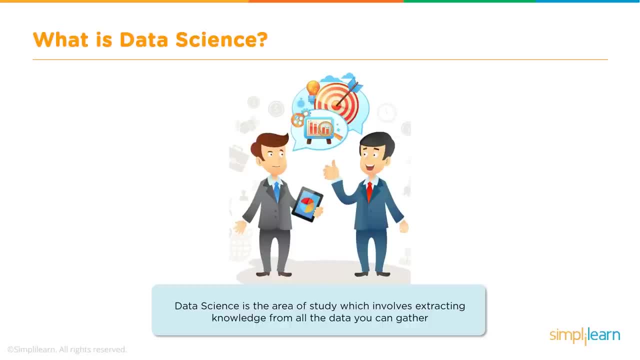 of using data and trying to find out some insights, or extracting some insights or knowledge using all the data that is at your disposal. so that's pretty much it what data science is all about. so you take the data and apply certain methodologies, certain algorithms and your business domain knowledge as well, and, of course, a certain amount of creativity. 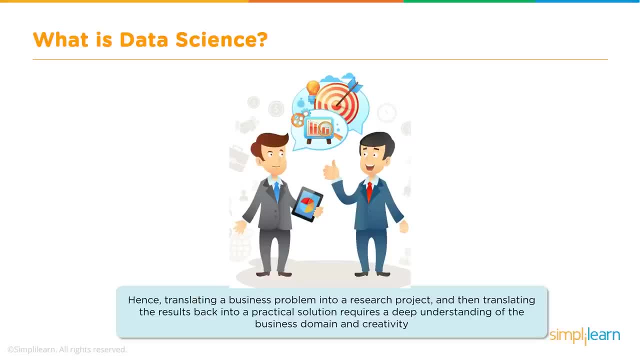 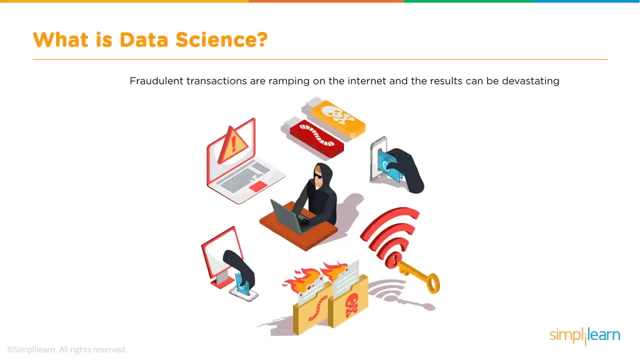 to extract some insights. very often they are also known as actionable insights, because once you have the insights, you should be in a position to take some action to, let's say, solve a problem or improve a situation. data science can be used. one of the very common one is fraud detection or fraud prevention. there 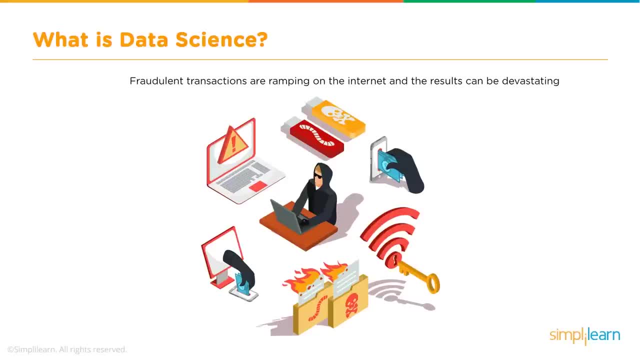 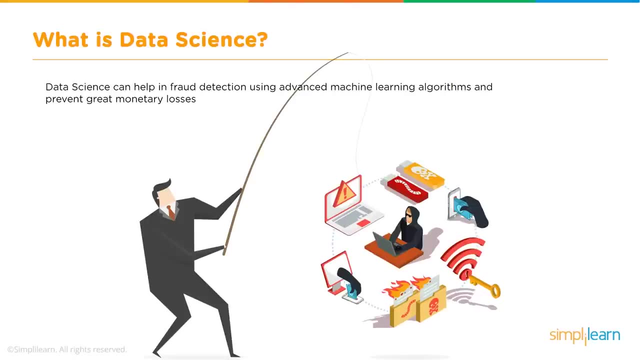 are a lot of fraudulent activities or transactions, primarily on the internet. it's very easy to commit fraud and therefore we can use data science to either prevent or detect fraud. there are certain algorithms- machine learning algorithms- that can be used, like, for example, some outlier techniques, clustering techniques- that can be used to detect fraud. 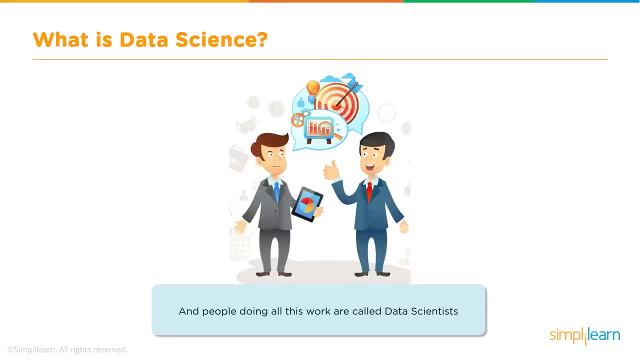 prevent fraud as well. so who is a data scientist? rather, it is actually a very generic role that defines. somebody who is working with data is known as a data scientist, but there can be very specific activities and the roles can be actually much more specific. what exactly a person does within? 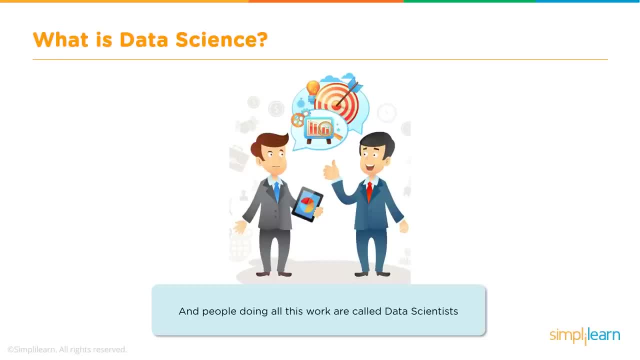 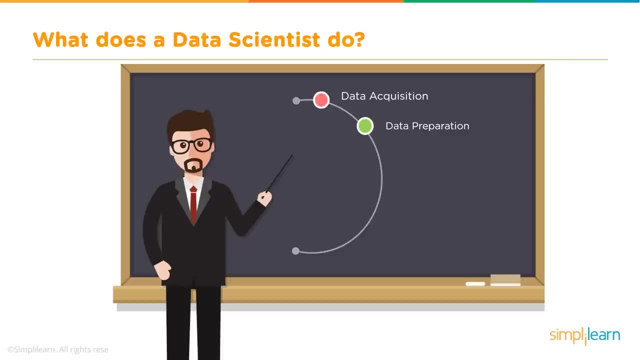 the area of data science can be much more specific, but broadly, anybody working in the area of data science is known as a data scientist. so what does a data scientist do? these are some of the activities: data acquisition, data preparation, data mining, data modeling and then model maintenance. we will talk about each of these in a great detail, but at a very high level. the 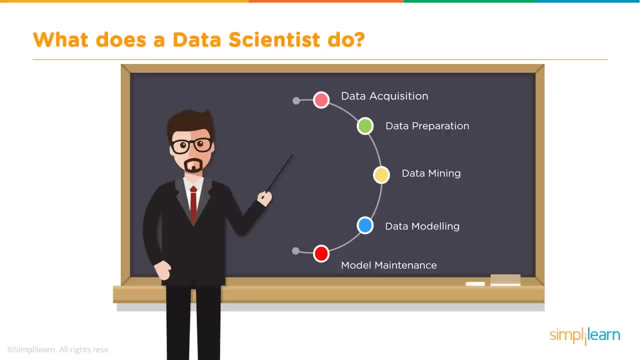 first step obviously is to get the raw data, which is known as data acquisition. it can be all kinds of format and it could be multiple sources, but obviously that raw data cannot be used, as it is, for performing data mining activities or data modeling activities. so the data has to be planned. 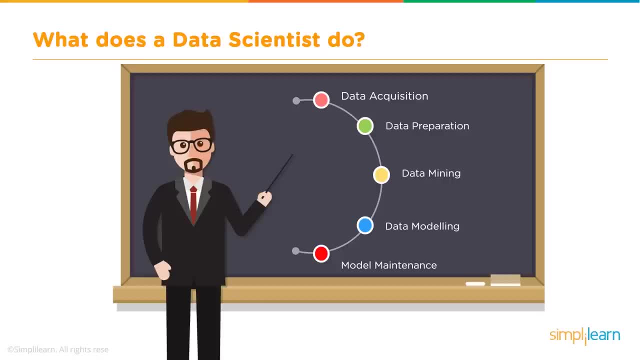 ahead for using in the data models or in the data mining activity. so that is the data preparation, then we actually do the data mining, which can also include some exploratory activities, and then if we have to do stuff like machine learning, then you need to build a machine learning model and test. 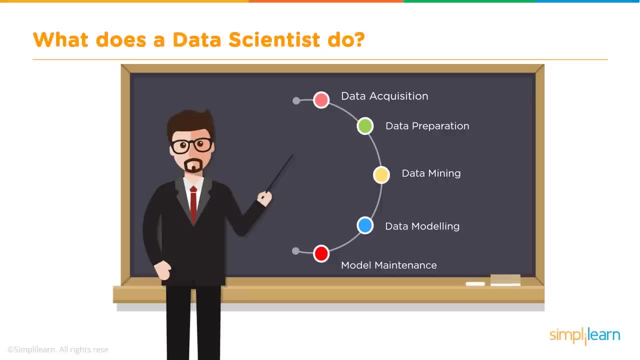 the model, get insights out of it, and then, if the model is fine, you deploy it. and then you need to maintain the model because over a period of time it is possible that you need to tweak the model because of change in the process or change in the data and so on, so that all comes under the model maintenance. so let's take deeper. 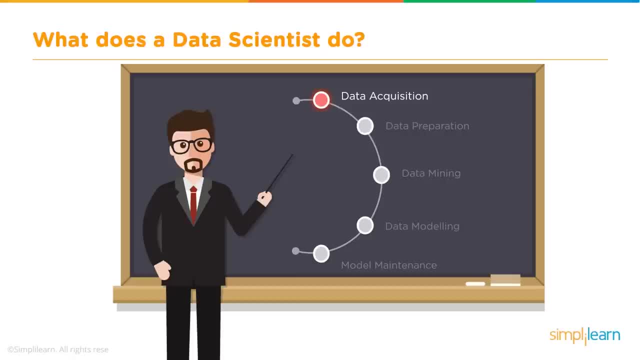 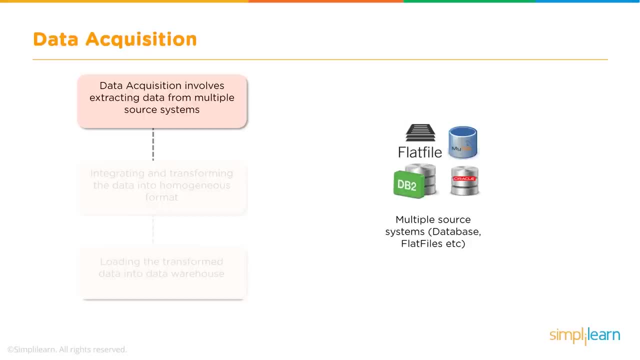 look at each of these activities. let's start with data acquisition. so the stage of data acquisition: basically, the data scientist will collect raw data from all possible sources. so this could be typically an rdbms, which is a relational database, or it can also be a non-rdbms or could be flat. 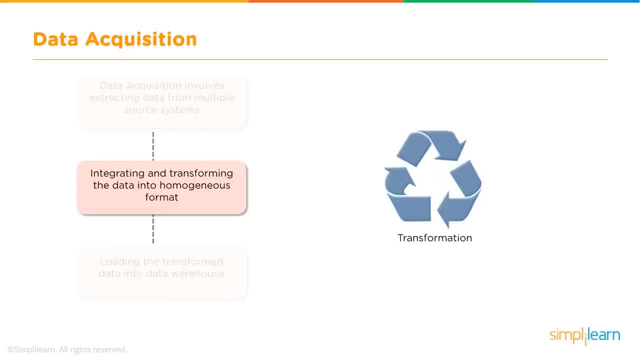 files or unstructured data and so on. so we need to collect all that data from different sources if required. we need to do some kind of homogeneous formatting so that it all fits into a in a looks at least- format. from a format perspective it looks homogeneous, so that may be requiring some kind of transformation. very often this is loaded into what 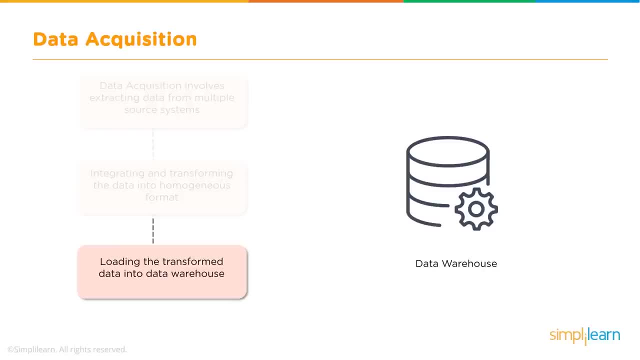 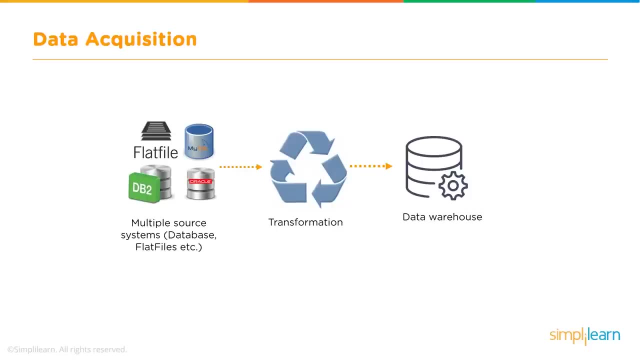 is known as data warehouse, so this can also be sometimes referred to as etl, or extract, transform and load. so our data warehouse is like a common place where data from different sources is brought together so that people can perform data science activities like reporting or data mining or statistical analysis and so on. so data from various sources. 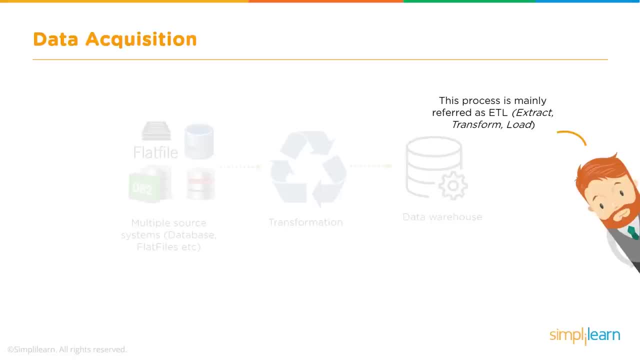 is put in a centralized place which is known as a data warehouse, so that is also known as etl, and in order to do this, there can be data scientists can take help of some etl tools. there are some existing tools that a data scientist can take help of, like, for example, data stage or talent. 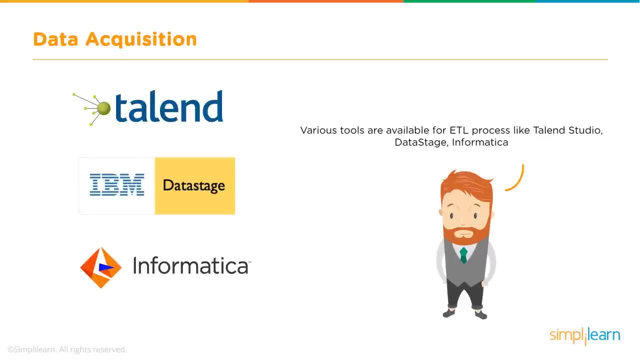 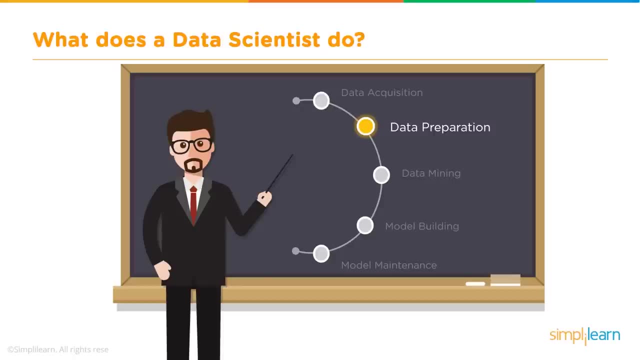 or informatica. these are pretty good tools for performing these etl activities and getting the data. the next stage, now that you have the raw data into a data warehouse, you still probably are not in a position to straight away use this data for performing the data mining activities. so that is. 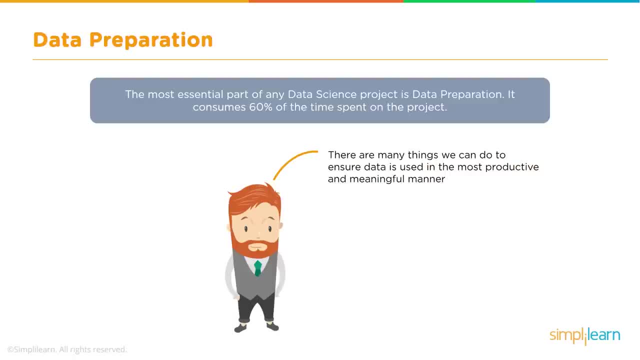 where data preparation comes into play, and there are multiple reasons for that. one of them could be: the data is dirty, there are some missing values and so on and so forth. so a lot of time is actually spent in this particular stage. so a data scientist spends a lot of time, almost 60 to 70 percent of 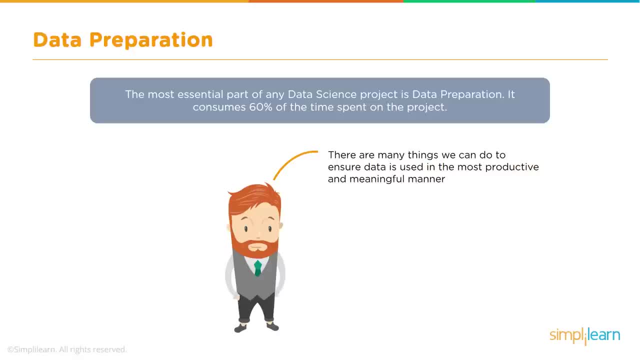 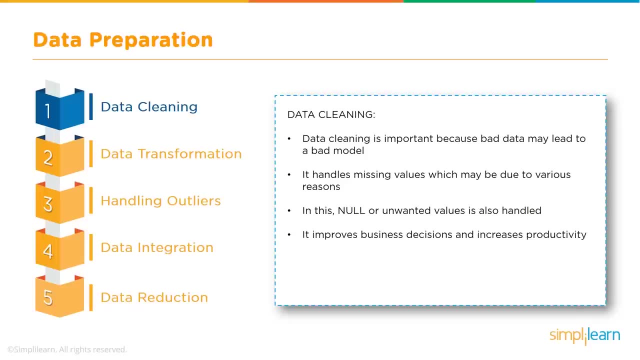 the time in this part of the project or the process, which is data preparation. so there are again within this, there can be multiple sub activities, starting from, let's say, data cleaning. you will probably have missing values, the data. there is some columns, the values are missing or the values are incorrect. 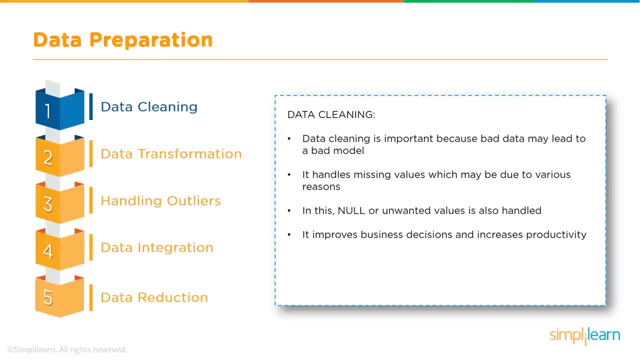 there are null values and so on and so forth. so that is basically the data cleaning part of it. then you need to perform certain transformations, like, for example, normalizing the data and so on. right, so you could probably have to modify a categorical values into numerical values and so on and so forth. so these are transformational. 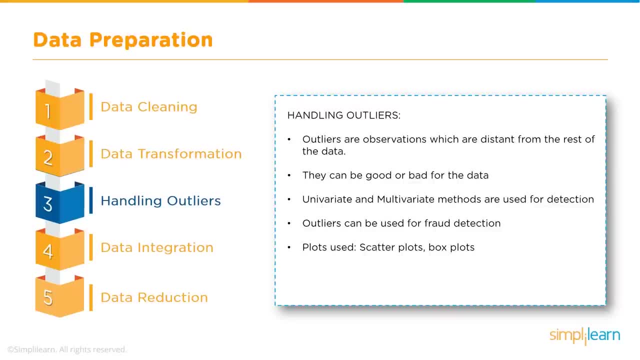 activities, then we may have to handle outliers. so the data could be such that there are a few values which are way beyond the normal behavior of the data, for whatever reason. either people have keyed in wrong values or for some reason some of the values are completely out of range, so those are known as outliers. so there are certain ways of handling these outliers. 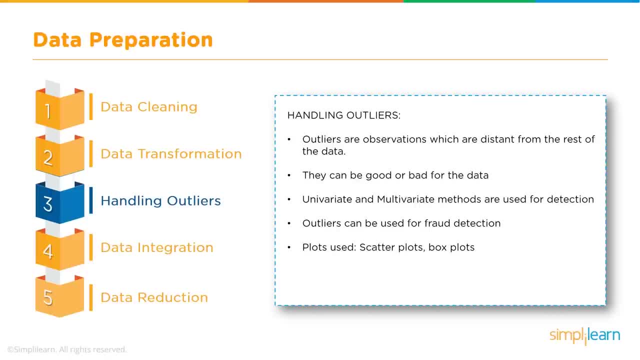 and detecting and handling these outliers. so this is a part of what is known as exploratory analysis, so you quickly explore the data to find out other so and you can use visual tools like plots and identify what are the outliers and see how we can get rid of the outliers and so on. then the next. 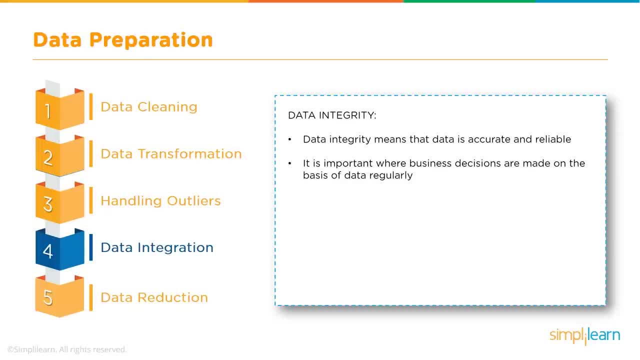 step is data integrity. data integrity is to validate, for example, if there are some primary keys, that all the primary keys are populated. there are some foreign keys, then at least most of the foreign keys should be populated, and otherwise, when we are trying to query the data, you might get wrong values and so on. so that is the data integrity part of it. and then we have 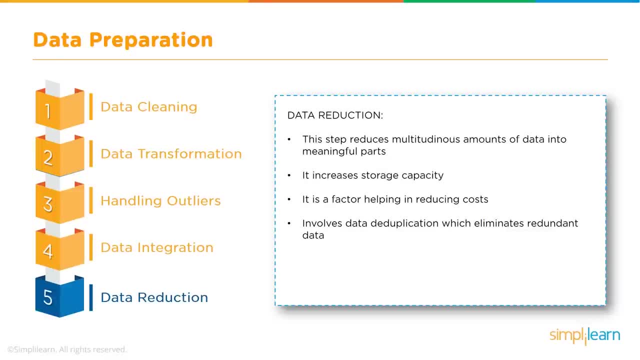 what is known as data reduction. sometimes we may have duplicate values, we may have columns that may be duplicated because they are coming from different sources, the same values are there, and so on. so a lot of this can be done using what is known as data reduction, and thereby you can reduce the size. 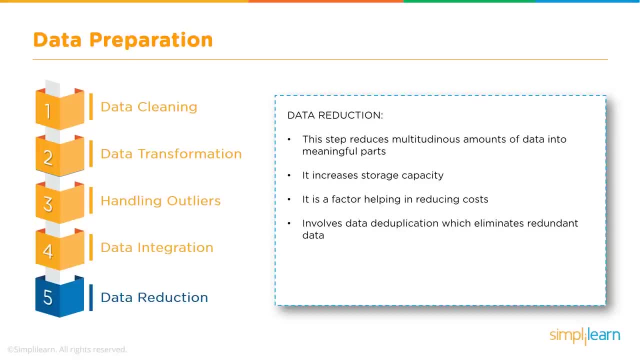 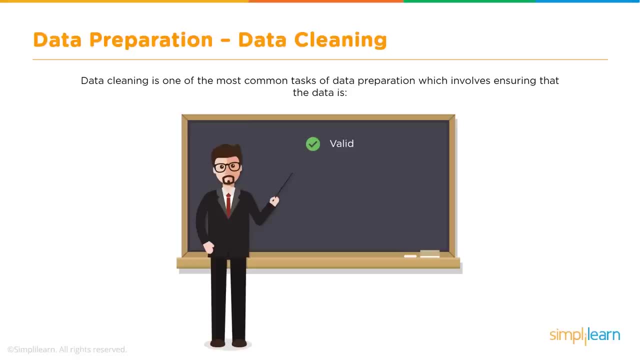 of the data drastically, because very often this could be written in data which can be removed and so on. so let's take a look at what are the various techniques that are used for data cleaning. so we need to ensure that the data is valid and it is consistent and uniform and accurate. so these are: 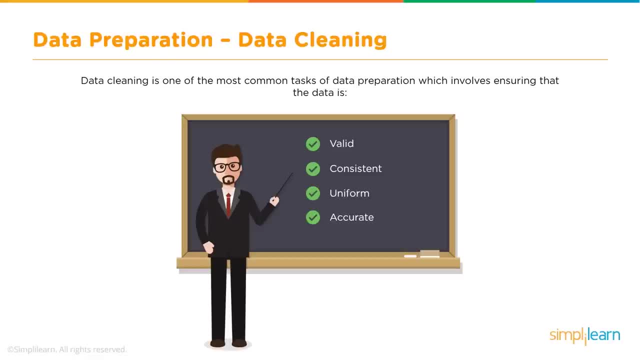 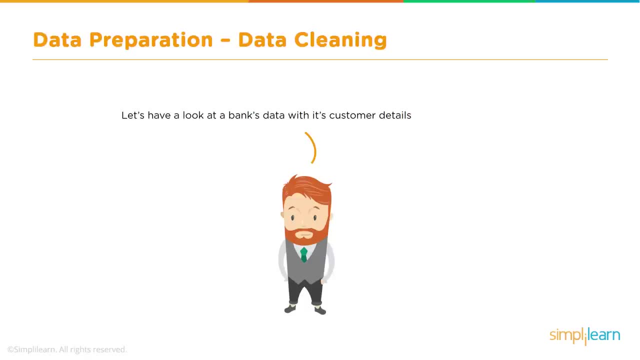 the various parameters that we need to ensure as a part of the data cleaning process. now, what are the techniques that that are used for data cleaning, or so we will see what each of these are in this particular case. and so what is the data set that we have? we have our data about a bank and its customer details, so let's take an. 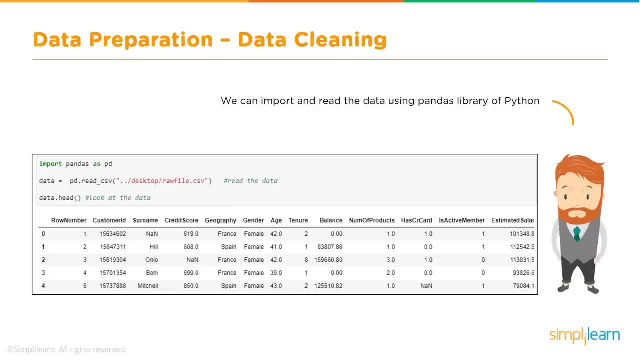 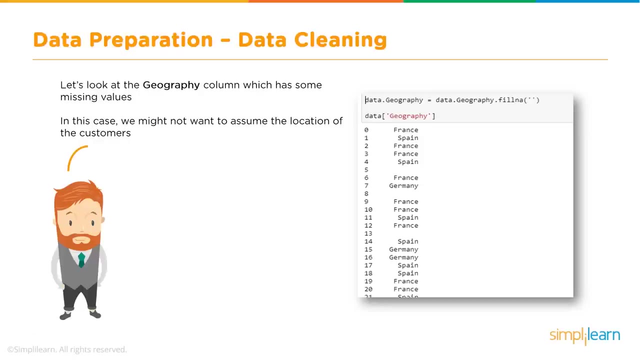 example and see how we go about cleaning the data. and in this particular example, we are assuming we are using python, so let's assume we loaded this data, which is the raw filecsv. this is how the customer data looks like and we will see. for example we take 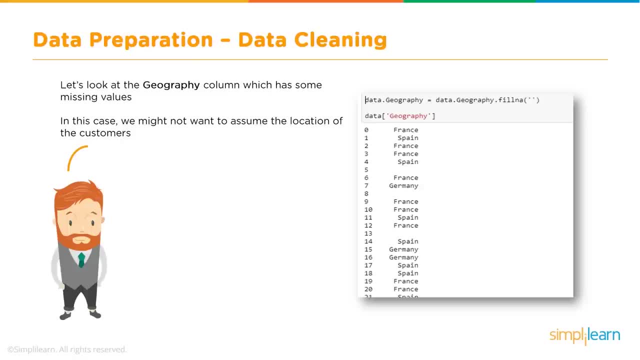 a closer look at the geography column, we will see that there are quite a few blank spaces. so how do we go about when we have some blank spaces? or if it is a string value, then we put a empty string here, or we just use a space or empty string if they are numerical values. 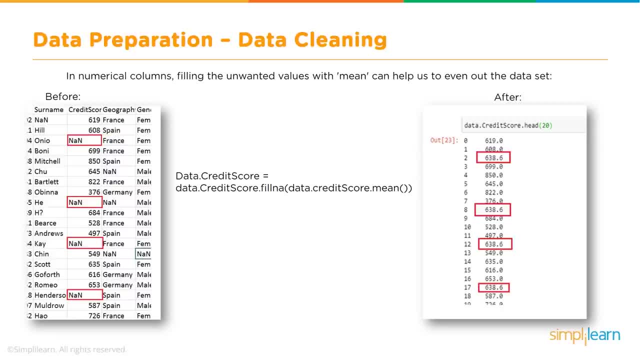 then we need to come up with a strategy. for example, we put the mean value. so wherever it is missing, we find the mean for that particular column. so in this case, let's assume we have credit score and we see that quite a few of these values are missing. so what do we do here? we find the mean. 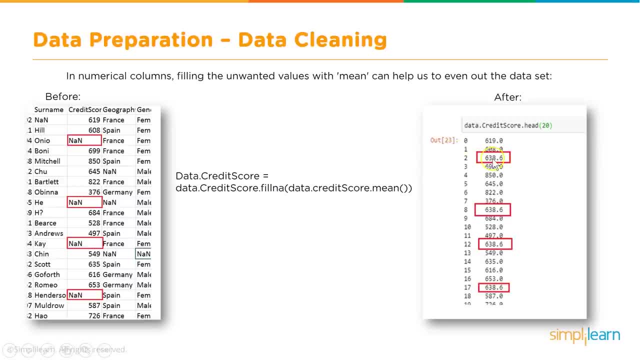 for this column for all the existing values, and we found that the mean is equal to 638.6. so we kind of use the piece of code to replace wherever there are blank values. nan is basically like null and we just go ahead and say: fill it with the mean value. so this is the piece of code we 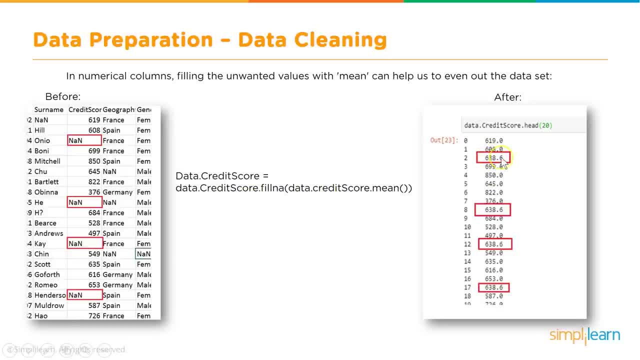 are writing to fill it. so all the blanks or all the null values get replaced with the mean value. now, one of the reasons for doing this is that very often, if you have some such situation, many of your statistical functions may not even work. so that's the reason you need to fill up these values, or? 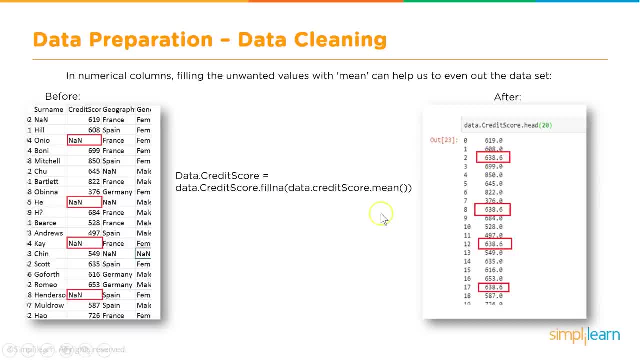 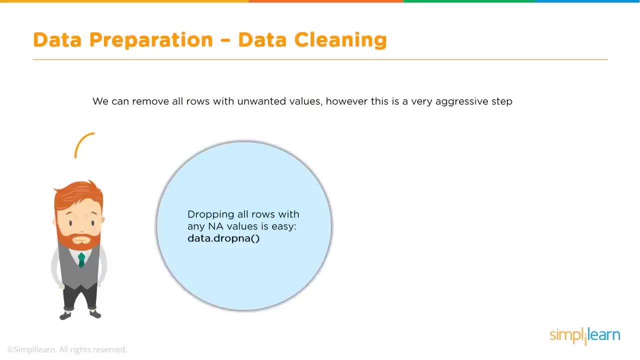 either get rid of these records or fill up these values with something meaningful. so this is one mechanism which is basically using a mean. there are a few others. as we move forward we can see what are the other ways. for example, we can also say that any missing value in a particular row, if even one column, the value is missing, you just drop that. 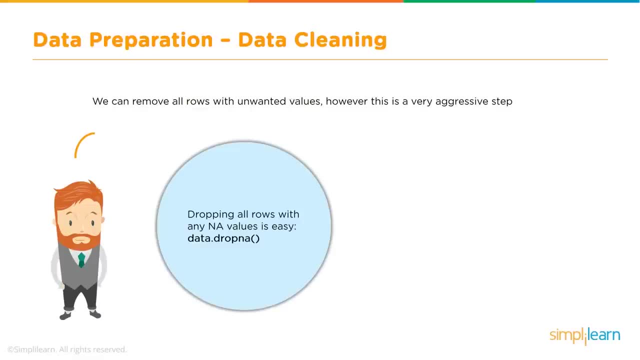 particular row or delete all rows where even a single column has missing values. so that is one way of dealing. now the problem here can be that if a lot of data has, let's say, one or two columns missing and we drop many such rows, then overall you may lose out on, let's say, sixty percent of the data. 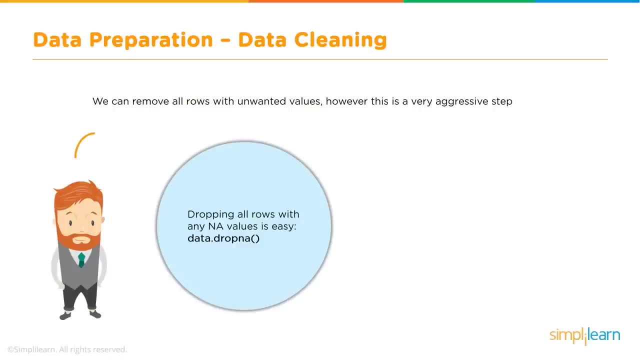 has some value or the other, missing sixty percent of the rows, then it may not be a good idea to delete all the rows like in that manner, because then you're losing pretty much sixty percent of your data. therefore your analysis won't be accurate. but if it is only five or ten percent, 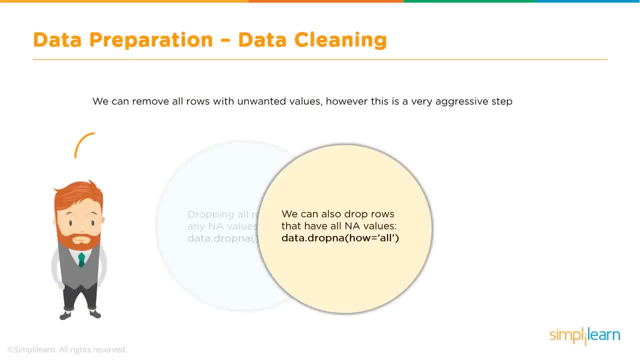 then this will work. another way is only to drop values where- or rather drop rows- where all the columns are empty, which makes sense, because that means that record is of really no use because it has no information in it. so there can be some situations like that. so we 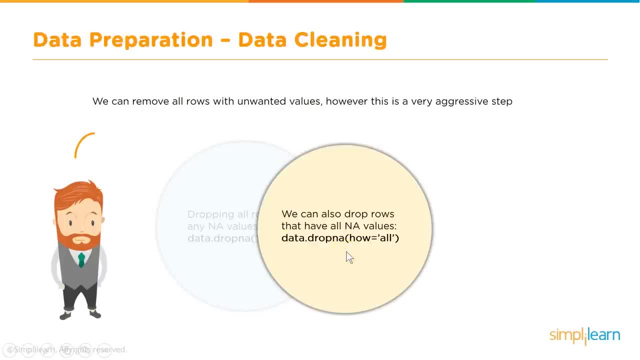 can provide a condition saying that drop the records where all the columns are blank or not applicable. we can also specify some kind of a threshold. let's say you have 10 or 20 columns in a row. you can specify that maybe five columns are blank or null. then you drop that record. so again. 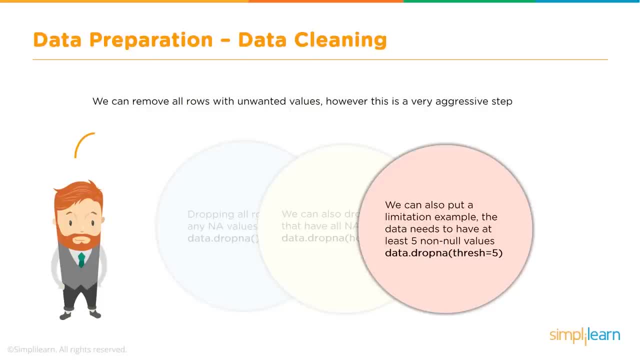 condition such a situation, the amount of data that has been removed or excluded is not large. if it is like maybe five percent, maximum ten percent, then it's okay. but by doing this, if you're losing out on a large chunk of data, then it may not be a good idea. you need to come up with. 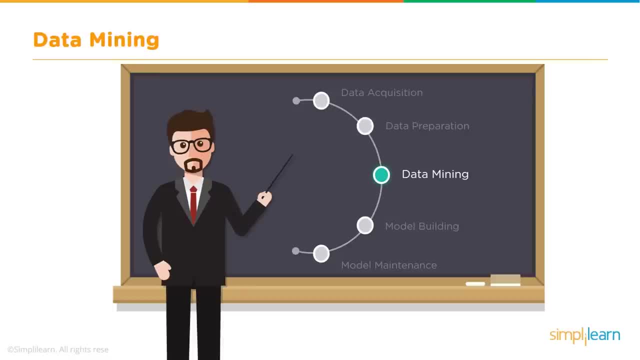 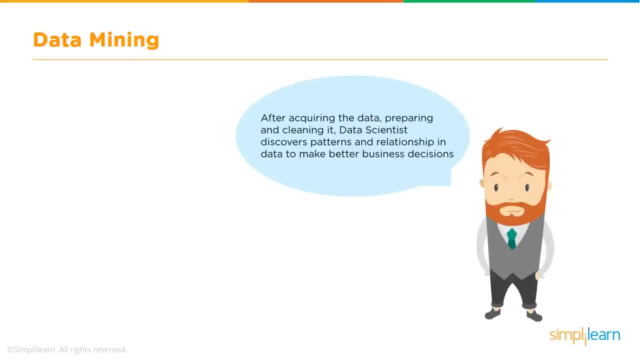 something better. what else we need to do next is so the data preparation part is done, so now we get into the data mining part. so what exactly we do in data mining? primarily, we come up with ways to take, take take a meaningful decisions. so data mining will give us insights into the data, what is existing there? 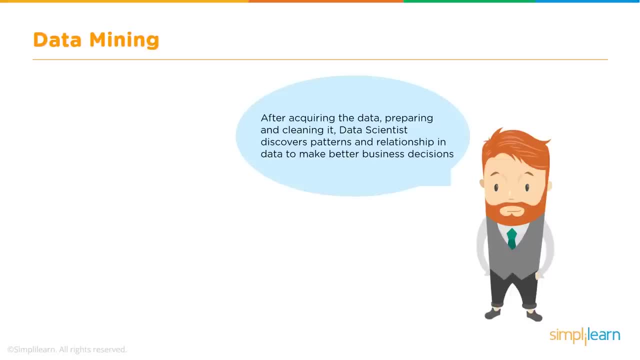 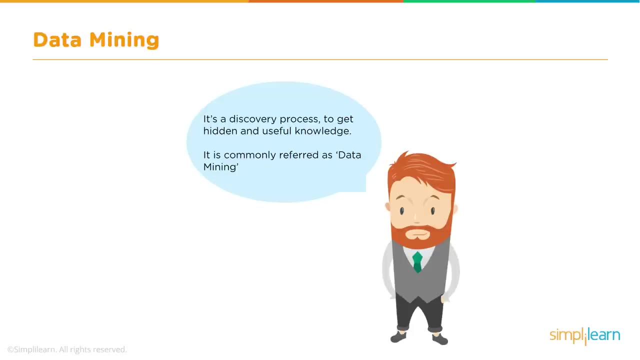 and then we can do additional stuff, like maybe machine learning and so on, to get perform advanced analytics and so on. so one of the first steps we do is what is known as data Discovery and uh, which is basically like exploratory analysis. so we can use tools like tableau for doing some. 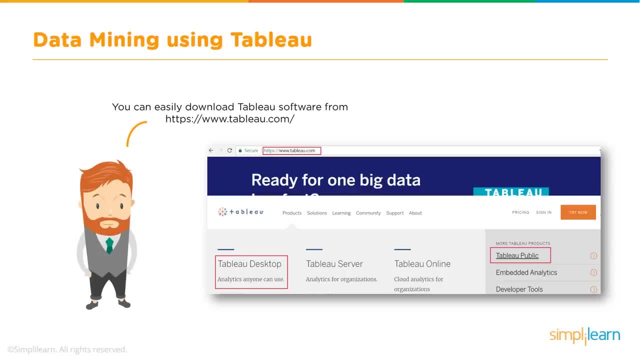 of this, so let's just take a quick look at how we go about that. so tableau is excellent data mining or actually more of a reporting or a bi tool, and you can download a trial version of tableau at tableaucom. or there is also tableau public, which is free and you can. 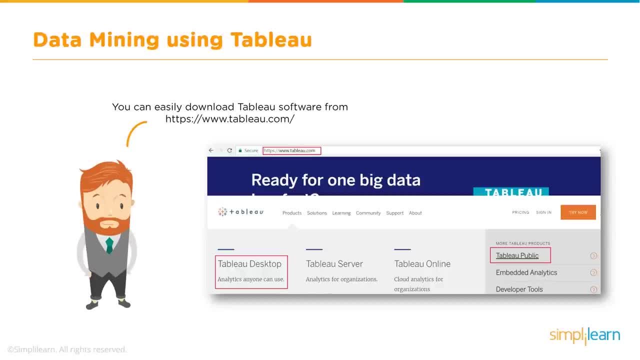 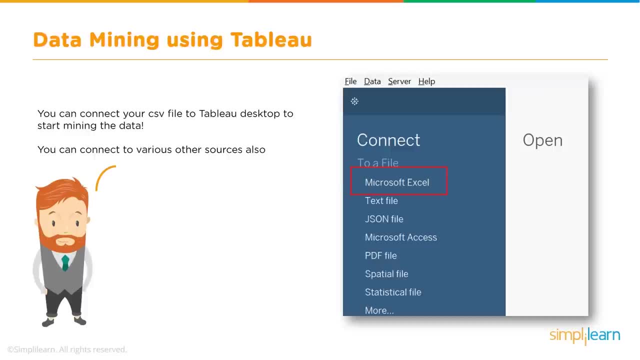 actually use and play around. however, if you want to use it for Enterprise purpose, then it is a commercial software, so you need to purchase license and you can then run some of the data mining activities. say, your data source. your data is in some excel sheet so you can select the source as microsoft, excel or any other format and the data 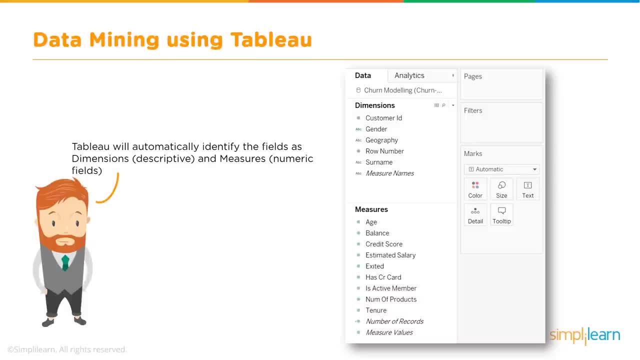 will be brought into the tableau environment and then it will show you what is known as dimensions and measures. so dimensions are all the descriptive columns, so and tableau is intelligent enough to actually identify these dimensions and measures. so measures are the numerical values. so, as you can see here- customer id, gender, geography- these are all dimensions, non-numerical values, whereas 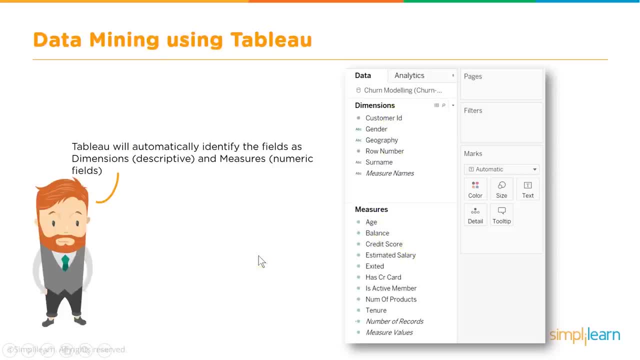 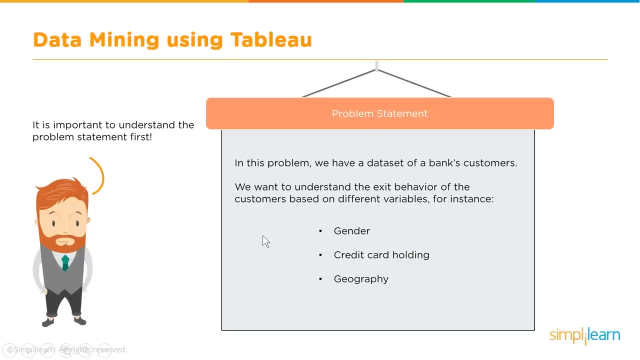 age, balance, credit score and so on are numeric values, so they come under measures. so you've got your data into tableau and then you want to, let's say, build a small model and you want to, let's say, a particular problem. so what is the problem statement? all right, let's say we want to analyze. 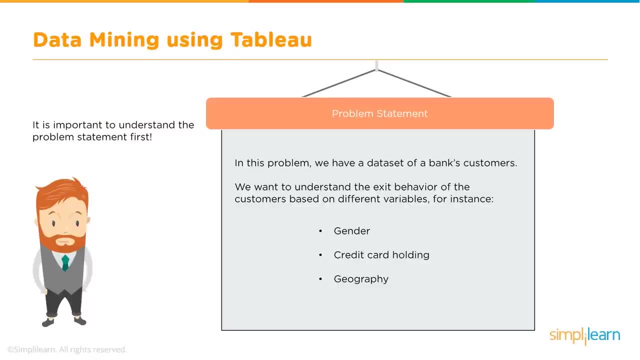 why customers are leaving the bank, which is known as exit, and we want to to analyze and see what are some of the factors for exiting the bank and we want to, let's assume, consider these three of them like, let's say, gender, credit card and geography, these as a criteria, and 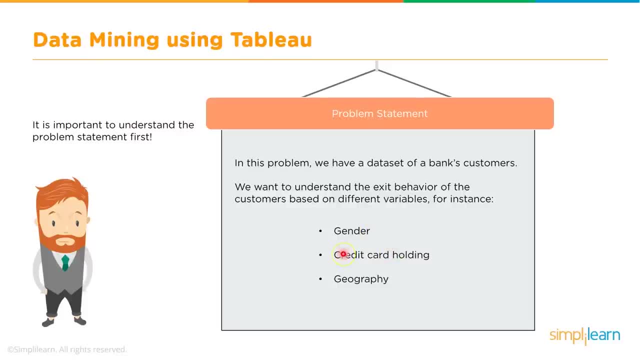 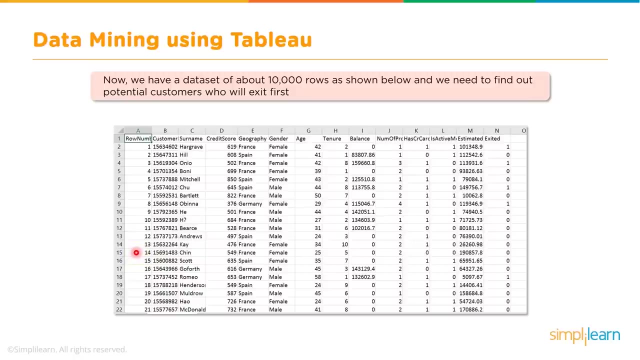 analyze if these are in any way impacting or have some bearing on the customer exiting or the customer exit behavior. okay, so let's use tab loop and very quickly we will be able to find out how these parameters are affecting. all right, so let's see. so this is our customer data. so from our Excel. 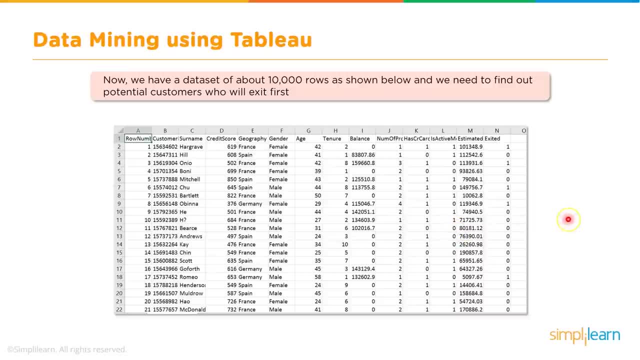 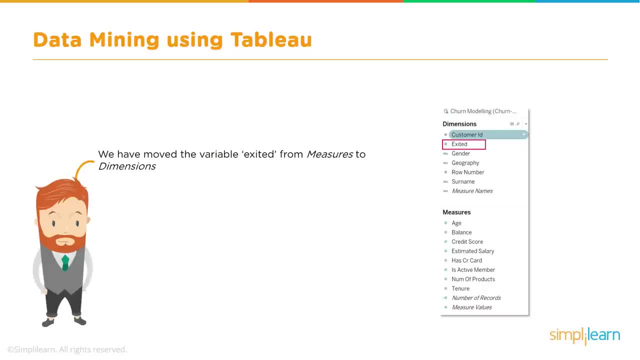 sheet. we have data set about, let's say, 10,000 rows and we want to find out what is the criteria. let's start with gender. let's say we want to first use gender as a criteria. so tableau really offers an easy drag-and-drop kind of a mechanism, so that makes it really really easy to perform this kind. 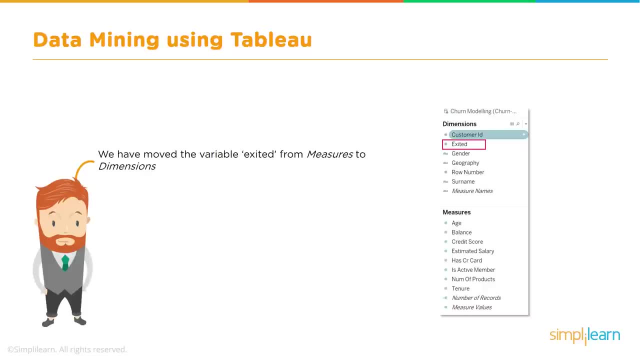 of analysis. so what we need to do is exit. it says whether the customer has exited or not, so it has a value of 0 and 1, and then, of course, you have gender and so on. so we will take these two and simply drag and drop. okay, so exit it, and then we will put gender, and if we 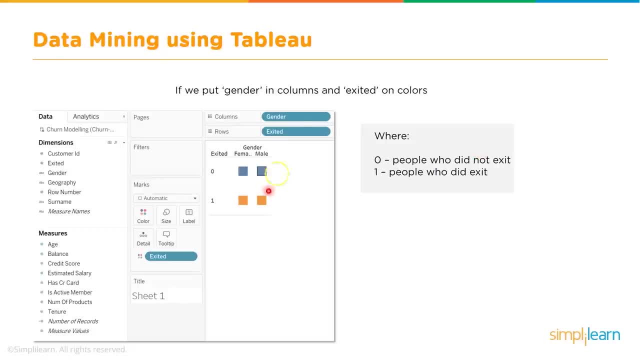 drag and drop into the analysis side of tab loop. alright, so here what we are doing is we are showing male, female as two different columns here, and zero for people who did not exist and one for people. blue color means people who did not exit and this yellow color means people who did exit. all right, 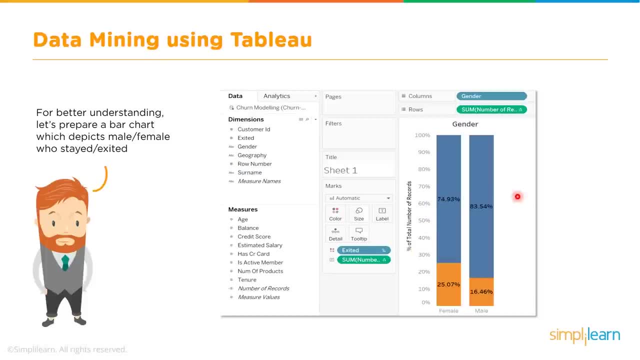 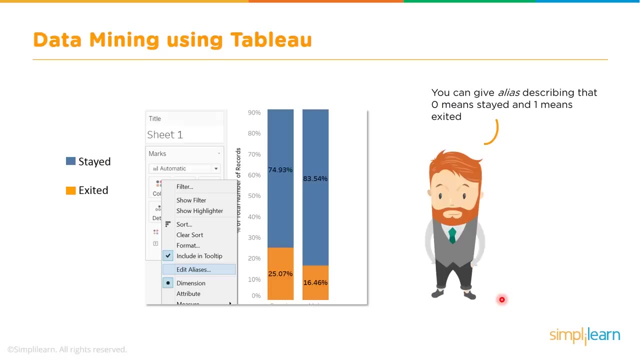 so now, if we pull the data here, create like bar graphs, this is how it would look. so what is yellow? let's go back. so yellow is who exited, and for the male, only 16.45 percent have exited, and we can also draw a reference line that will help us or even provide aliases. so these are a lot of fancy stuff. 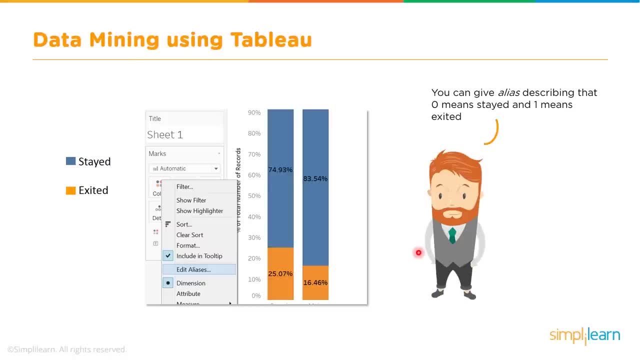 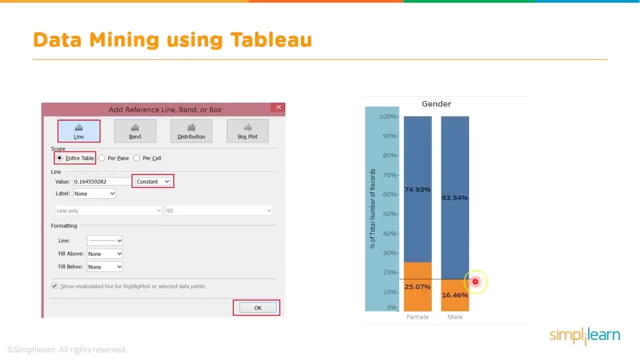 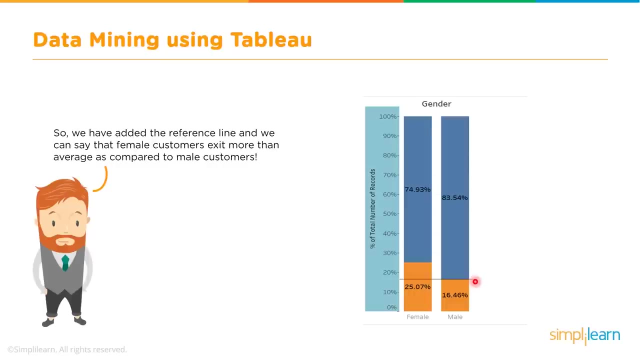 in tablo, you can create aliases and so that it looks good rather than basic labels, and you can also add a reference line. so you add a reference line, something like this: from here we can make out that, on an average, female customers exit more than the male customers. right, so that is what we 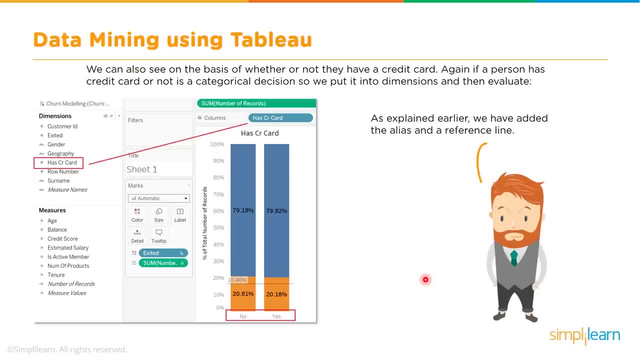 are seeing here on an average. so we have analyzed based on gender. we do see that there is some difference in the male and female behavior. now let's take the next criteria, which is the credit card. so let's see if having a credit card has any impact on the customer exit behavior. 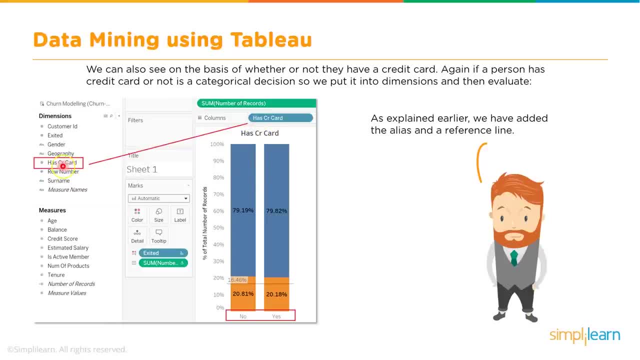 so, just like before we drag and drop the credit card, has credit card a column. if we drag and drop here and then we will see that there is pretty much no difference between people having credit card and not having credit card. 20.81 of people who have no credit card have exited and similarly. 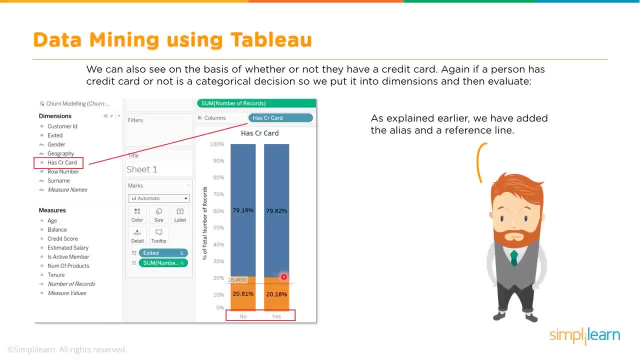 20.18 percent of people who have credit card have also exited. so the credit card having credit card also absensibility is seen that by having a credit card and not having credit card- for example, in pr democracy credit cards compare three different 500 pesos each. that doesn't mean that you don't have credit card. that 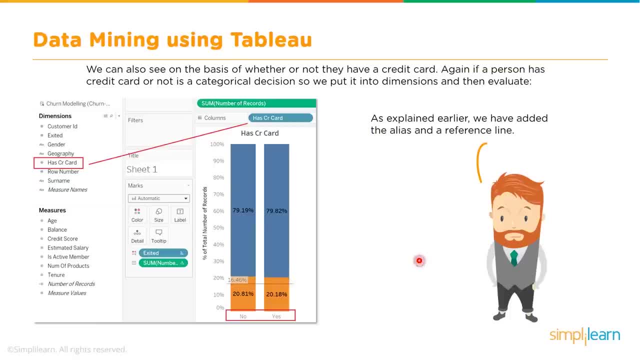 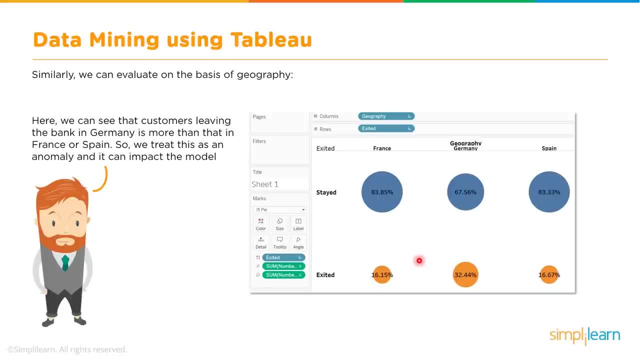 card is not having much of an impact. that's what this piece of analysis shows. last, we will basically go and check how the geography is impacting. so once again, we can drag and drop geography column on to this side and if we see, here there are geographies like I think there are about three geographies. 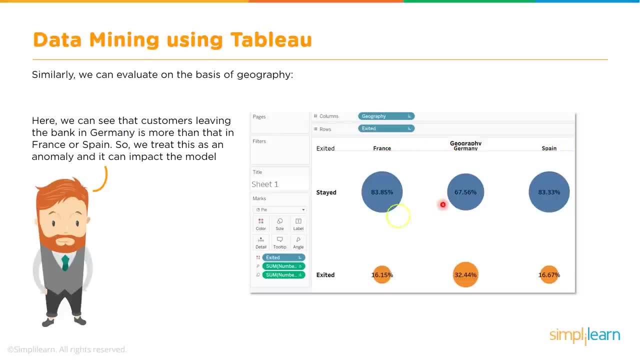 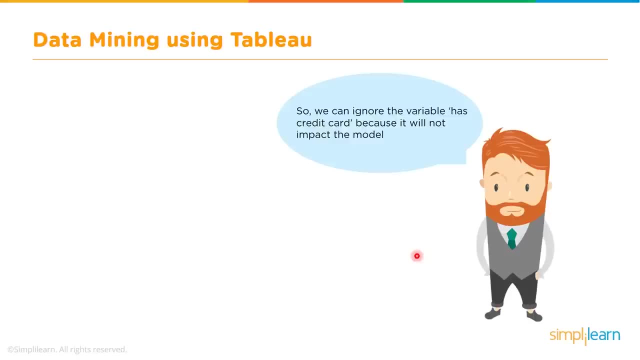 like France, Germany and Spain, and we see that there is some kind of impact with the geography as well. okay, so what we derive from this is that the credit card is really. we can ignore the credit card variable or feature from our analysis because that doesn't have any impact, but gender and geography we can keep and do. 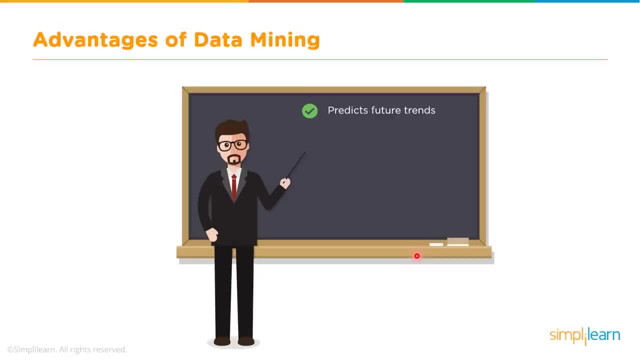 further analysis. okay, all right. so what are some of the advantages of data mining bit? more detailed analysis can help us in predicting the future trends and it also helps in identifying customer behavior. you patterns. okay, so you can take informed decisions because the data is telling you or providing you with some insights, and then you take decision based on that. 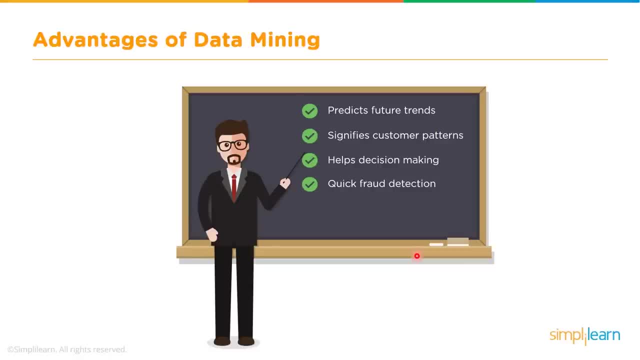 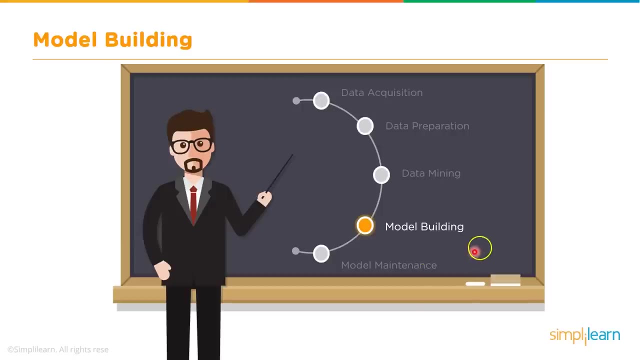 if there is any fraudulent activity. data mining will help in quickly identifying such a fraud as well, and, of course, it will also help us in identifying the right algorithm for performing more advanced data mining activities, like machine learning and so on. all right, so the next activity, now that we have the 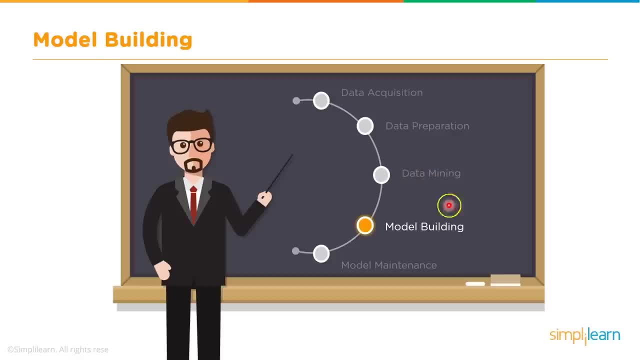 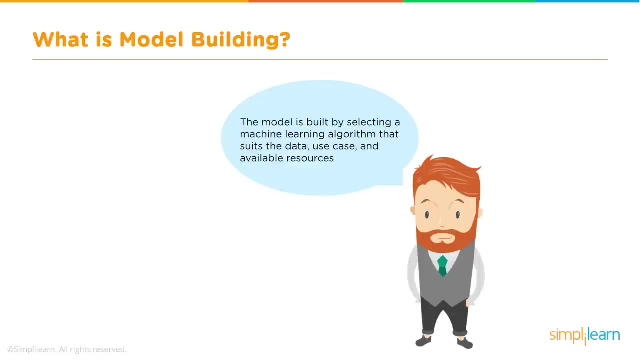 data- we have here the data- and perform some data mining activity. the next step is model building. let's take a look at model building. so what is a model building? if you want to perform a more detailed activity, like maybe perform some machine learning, then you need to build a model. 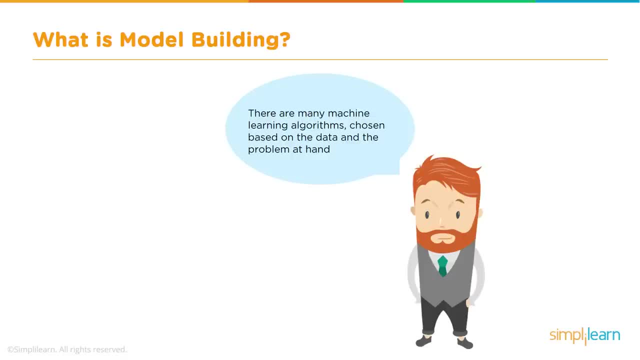 and how do you build a model? first thing is you need to select which algorithm you want to use to solve the problem on hand, and also what kind of data that is availableann you want to know to solve a problem on hand, so you need to use a. 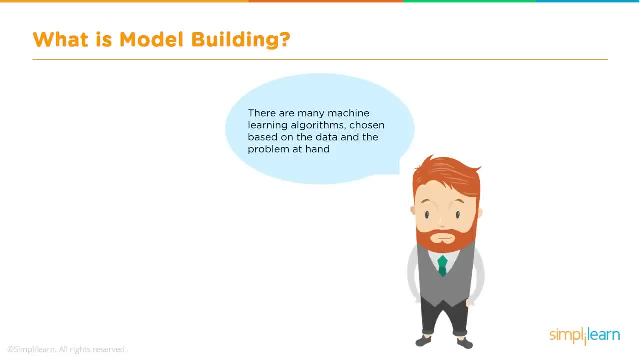 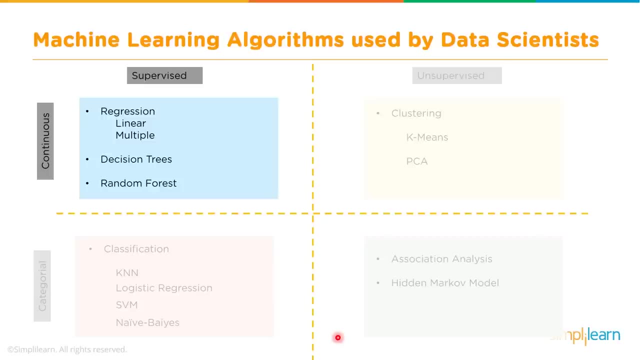 so on and so forth. so you need to make a choice of the algorithm and based on that you go ahead and create a model, train the model and so on. now machine learning is kind of at a very high level, classified into supervised and unsupervised. so if we want to predict a continuous value- could be a price or a- 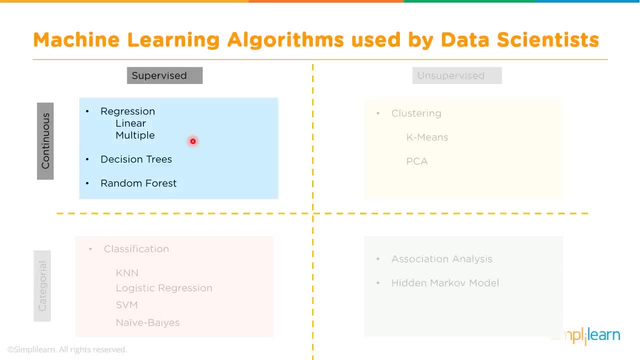 temperature or a height or a length, things like that. so those are continuous values and if you want to find some of those, then you use techniques like regression, linear regression, simple linear regression, multiple linear regression, and so on. so these are the algorithms. on the other hand, there will 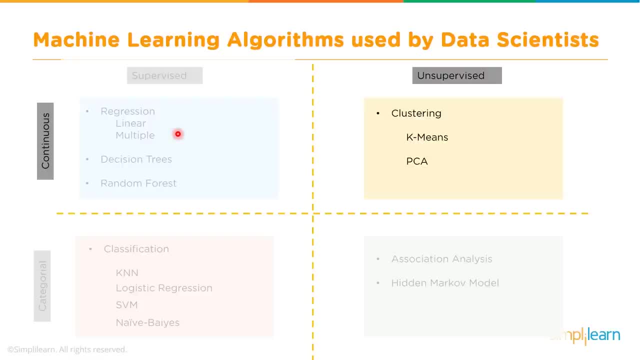 be situations. so there may be situations where you need to perform unsupervised learning. case of unsupervised learning: you don't have any historical labeled data so to learn from. so that is when you use unsupervised learning and some of the algorithms in unsupervised learning are clustering. K means 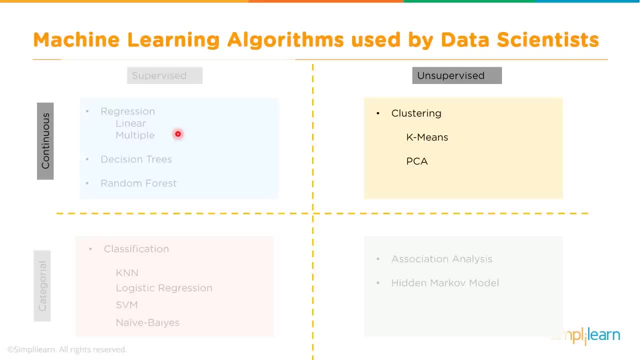 clustering is the most common algorithm used in unsupervised learning, supervised learning and similarly in supervised learning. if you want to perform some activity on categorical values like, for example, it is not measured but it is counted, like you want to classify whether this image is a cat or a dog, whether you want to classify whether this customer 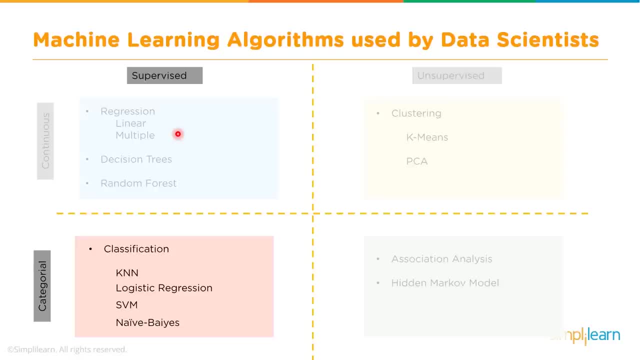 will buy the product or not, or you want to classify whether this email is spam or not spam. so these are examples of categorical values and these are examples of classification. then you have algorithms like logistic regression, k, nearest neighbor or knn and support vector machine. so these are some of the algorithms that are used in this case and similarly in case of unsupervised 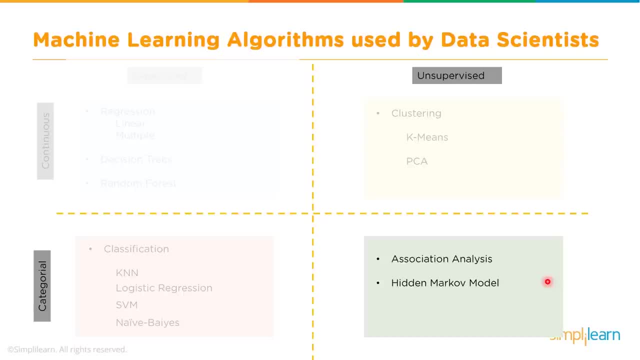 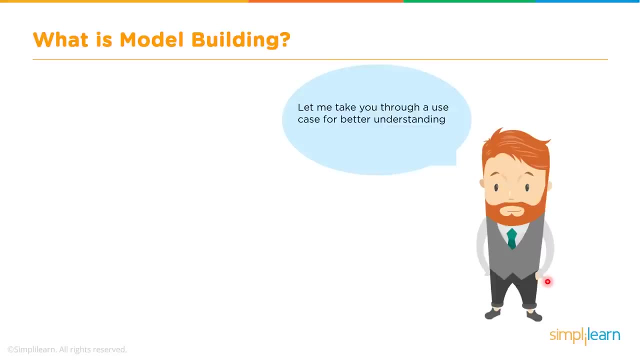 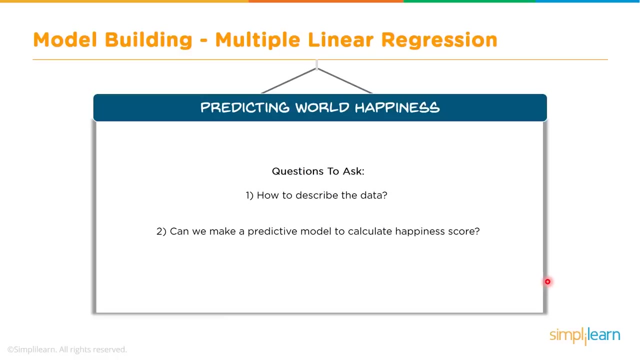 learning. if you need to perform on categorical values, you have some algorithms like association analysis and hidden marco model. okay, so in order to understand this better, let's take an example and take you through the whole process, and then we will also see how the code can. 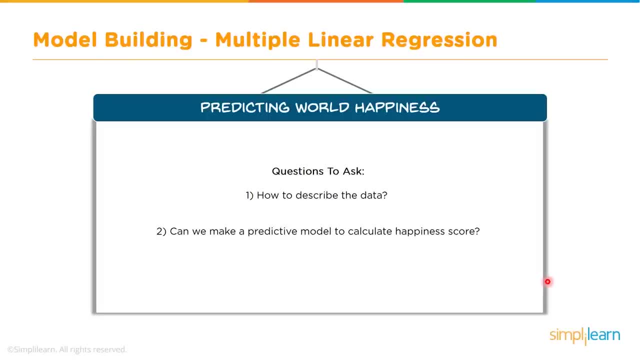 be used in this case. so let's take an example and take you through the whole process, and then we will also see how the code can be used in this case, written to perform this. now let's take our example here, where we want to perform a supervised learning. 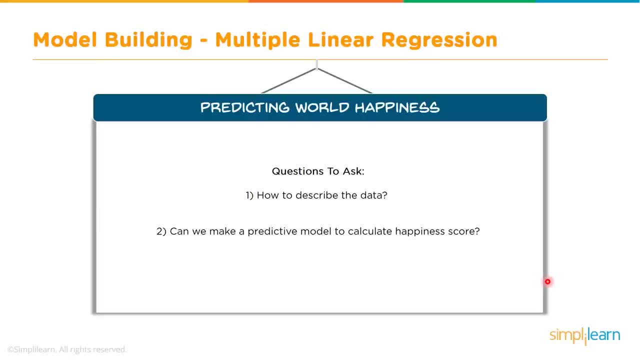 which is basically we want to do a multi-linear regression, which means there are multiple independent variables, and then we want to perform a linear regression to predict certain value. so in this particular example, we have world happiness data, so this is the data about the happiness quotient of people from various countries and we are trying to predict and see whether our 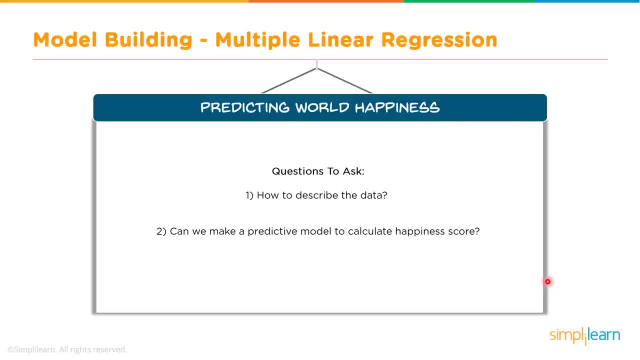 how our model will perform. so what is the? this is the question that we need to ask: first of all, how to describe the data, and then can we make a predictive model to calculate the happiness score right? so based on this, we can then decide on what algorithm to use and what model to use. 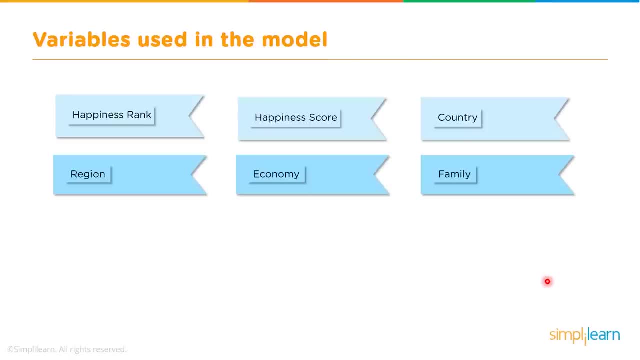 and so on. so variables that are available are used in this model. this is a list of variables that are available. there is a happiness rank. I'll load the data and or I'll show you the data in a little bit so it becomes clear what are these. so there is what is known as a happiness rank- happiness score. 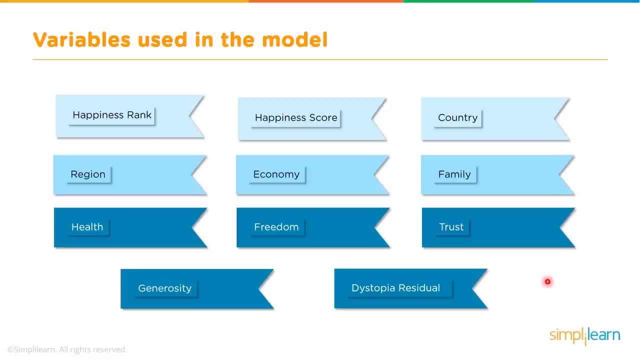 which is happiness. score is more like absolute value, whereas rank is: what is the ranking? and then which country we are talking about and within that country, which region and what kind of economy, and whether the family, which family and health, details and freedom, trust, generosity and so on. 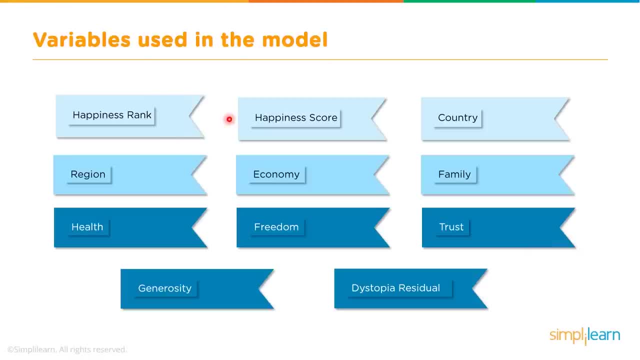 and so forth. so there are multiple variables that are available to us and the specific details probably are not required, and there can be in another example the variables can be completely different. so we don't have to go into the details of what exactly these variables are, but just 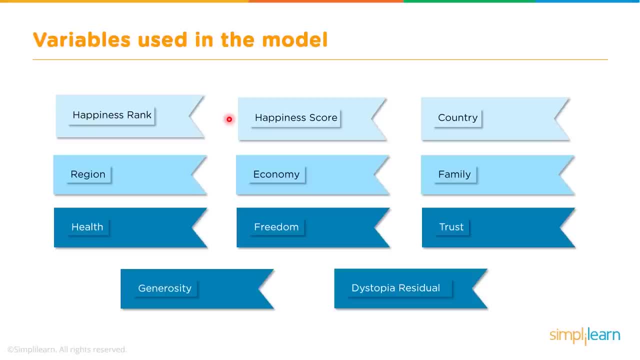 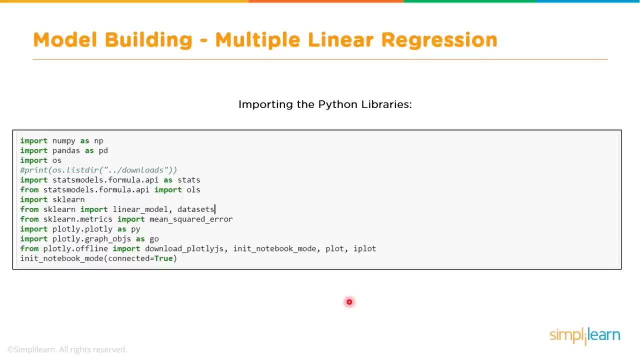 enough to understand that we have a bunch of these variables and now we need to use either all or some of these variables and then, which we also sometimes refer to as features, and then we need to build our model and train our model. all right, so let's assume we will use python in order to 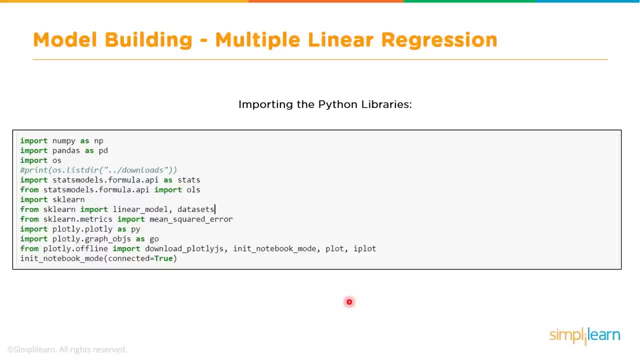 perform this analysis or perform this machine learning activity, and i will actually show you, in our lab in in a little bit, this whole thing. we will run the live code, but quickly. i will run you through the slides and then we will go into the lab. so what are we doing here? first thing we need to do: 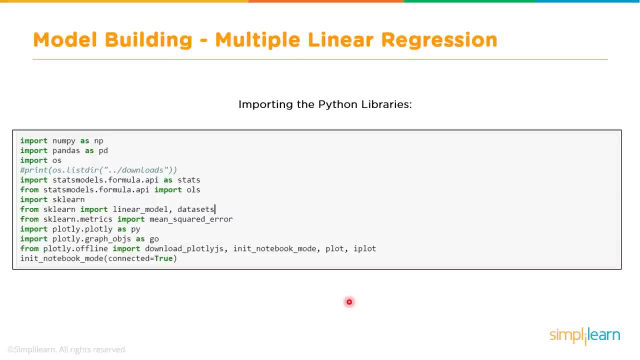 is import a bunch of libraries in python which are required to perform our analysis. most of these are for manipulating the data, preparing the data, and then scikit-learn or sklearn is the library which we will use actually for this particular machine learning activity, which is linear regression. so 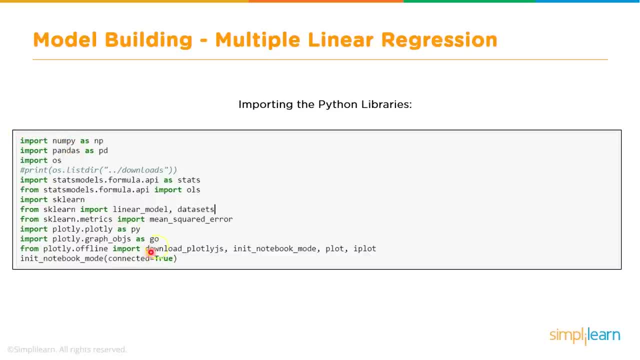 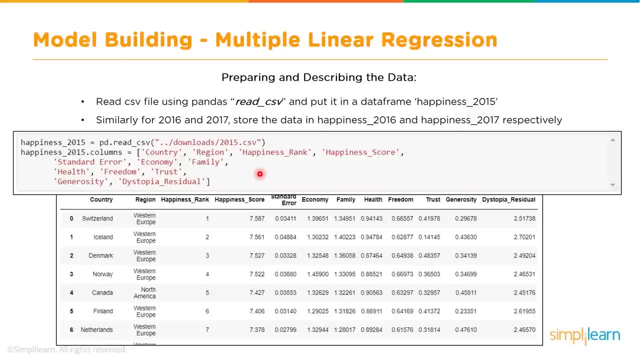 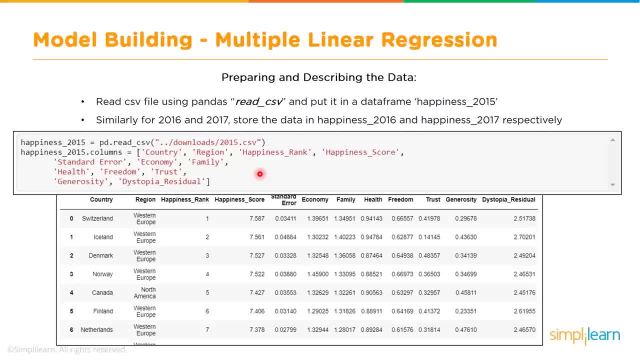 have data for 2015, 16 and 17, and so we will load this data and then combine them, concatenate them to prepare a single data frame. and here we are making an assumption that you are familiar with python, so it becomes easier if you are familiar with python programming language. 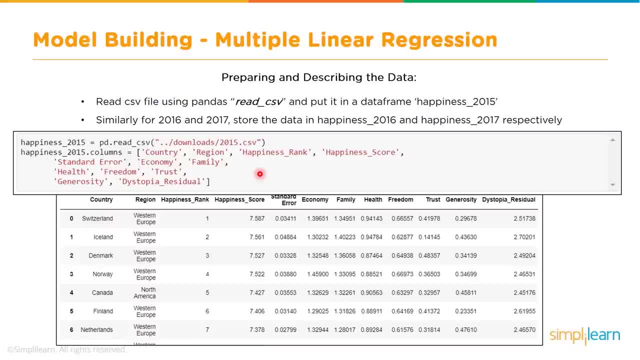 or at least some programming language, so that you can at least understand by looking at the code. so we are reading the file, each of these files for each year, and this is basically. we are creating a list of all the names of the columns we will be using later on. you will see in the code. so we have 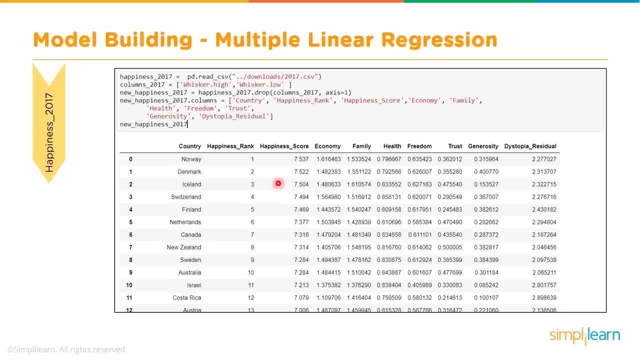 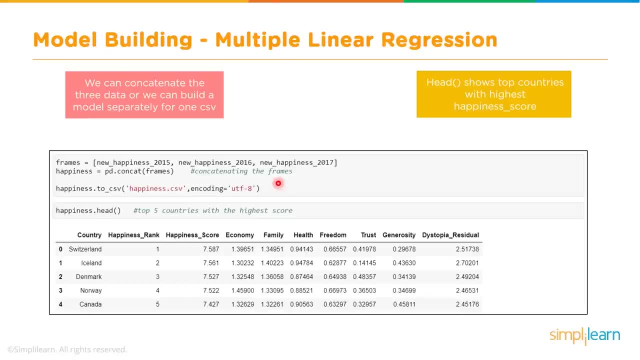 loaded 2015, then 2016 and then also 2017.. so we have created three data frames and then we concatenate all these three data frames. this is what we are doing here. then we identify which of these columns are required. which, for example, some of the categorical values do we really need? we 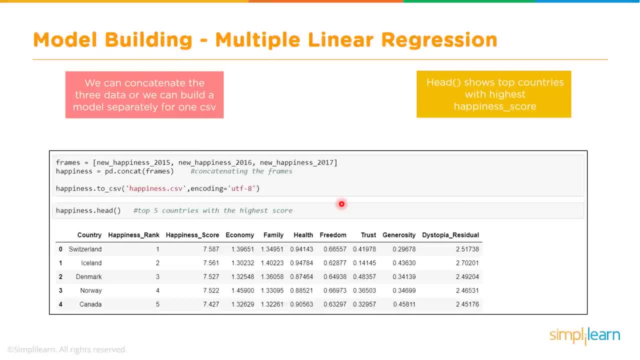 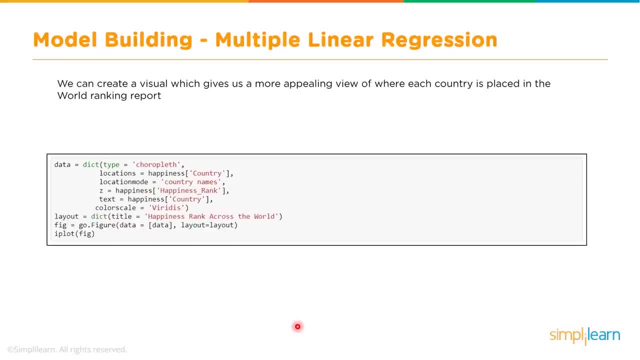 probably don't, then we drop those columns so that we don't unnecessarily use all the columns and make the computation complicated. we can then create some plots using plotly library, and it has some powerful features, including creation or creation of maps and so on. just to understand the 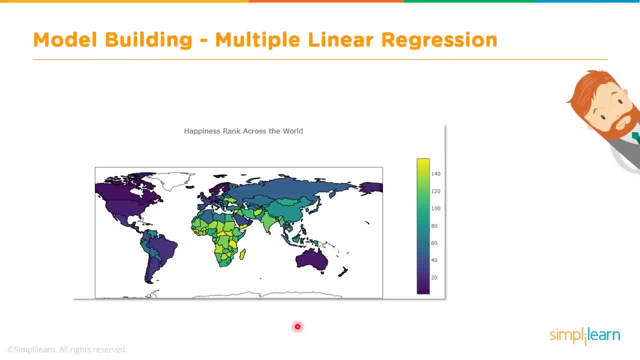 pattern, the happiness quotient, or how the happiness is across all the countries. it's a nice visualization. we can see each of these countries how they are in terms of their happiness score. this is the legend here. so the lighter colored countries have lower ranking, and so these are the lower ranking ones and these are higher ranking, which means that the ones with these 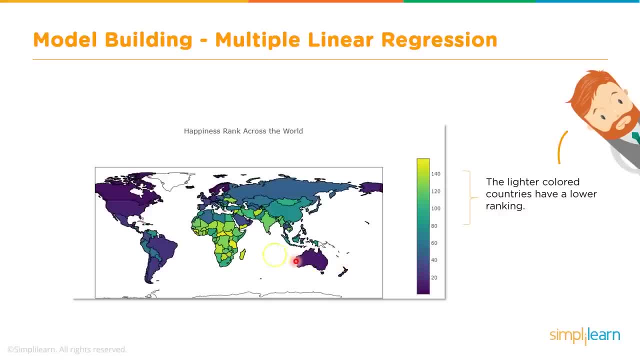 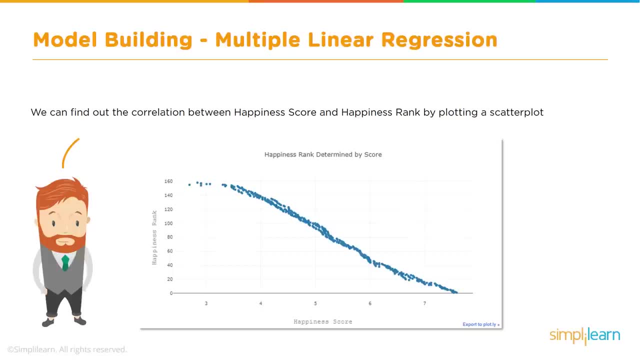 dark colors are the happiest ones. so, as you can see here, australia, and maybe this side- uh, us and so on- are the happiest ones. okay, the other thing that we need to do is the correlation between the score and happiness rank. we can find a correlation using a scatter plot and we find that, yes, they are. 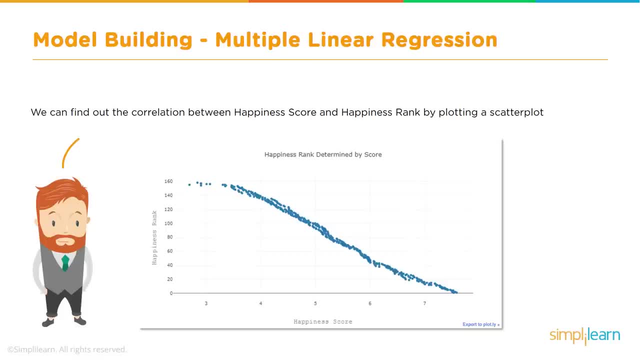 kind of inversely proportion, which is obvious. so if the score is high, happiness score is high, then they are ranked number one. for example, highest is scored as number one. so that's the idea behind this. so the happiness score given here and the happiness rank is actually given here. so they 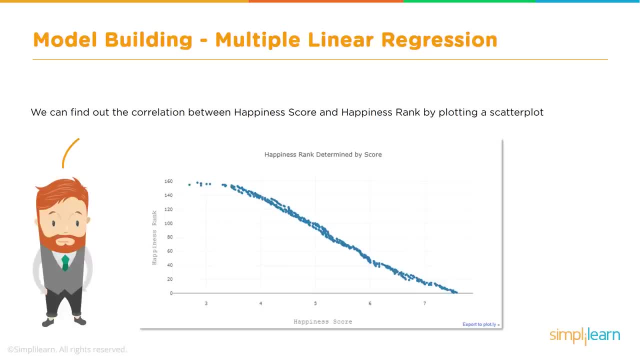 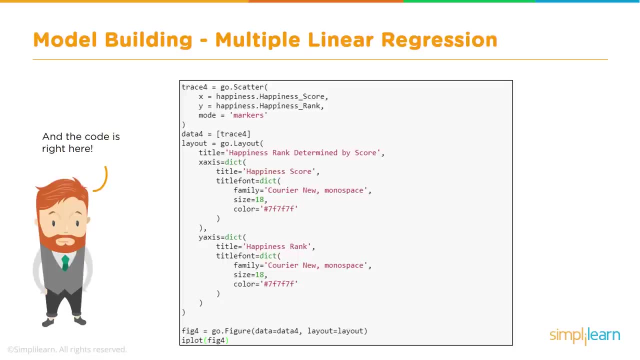 are inversely proportional, because the higher the score, the absolute value of the rank will be lower. number one has the highest value of the score, and so on. so they are inversely correlated, but there is a strong. what this graph shows is that there is a strong correlation between happiness rank and 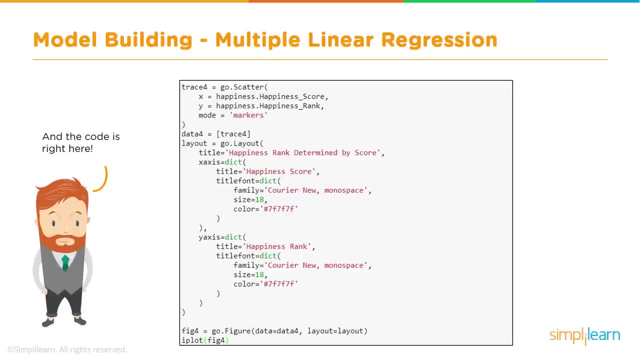 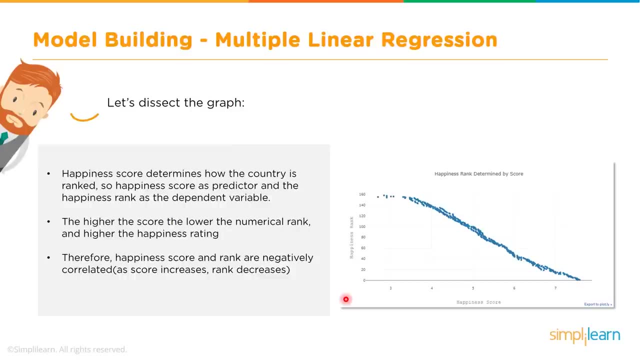 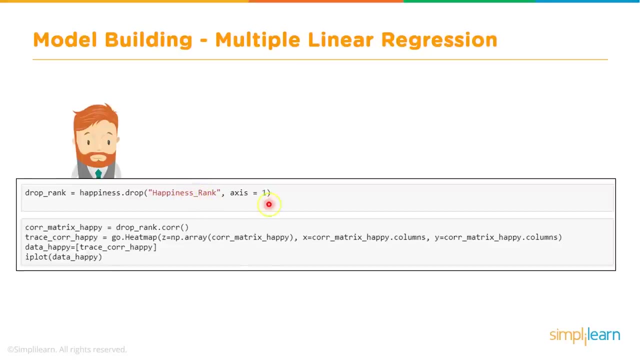 happiness score. and then we do some more plots to visualize this. we determine that probably rank and score are pretty much conveying the same message, so we don't need both of them. so we will kind of drop one of them, and that is what we are doing here. so we drop the happiness rank and similarly. 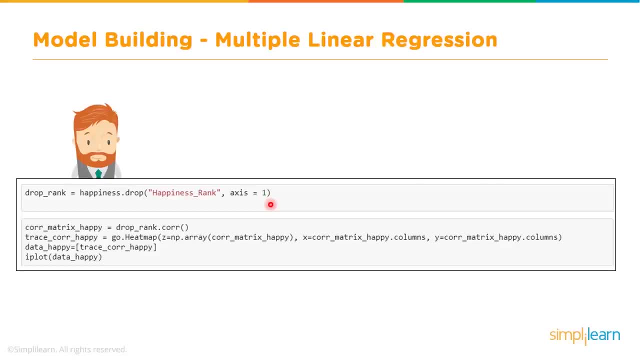 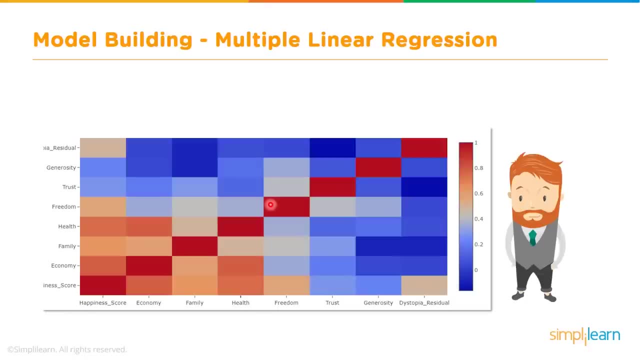 this is one example of how we can remove some columns which are not adding value, so we will see in the code as well how that works. moving on, this is a correlation between pretty much each of the columns with the other columns. so this is a correlation you can plot using plot function. 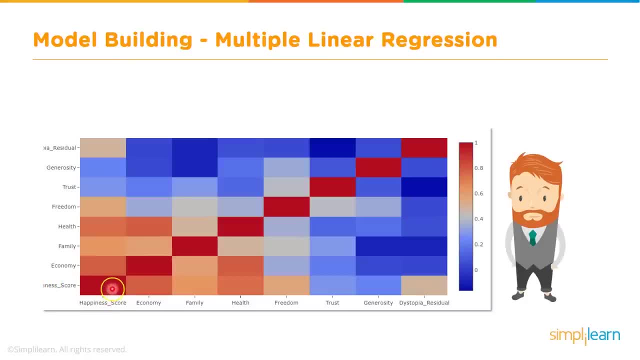 and we will see here that, for example, happiness score and happiness score are correlated. strongest correlation, right, because every variable will be highly correlated to itself. so that's the reason why it is called a correlation. so the higher the color is, the higher the correlation, and as so the 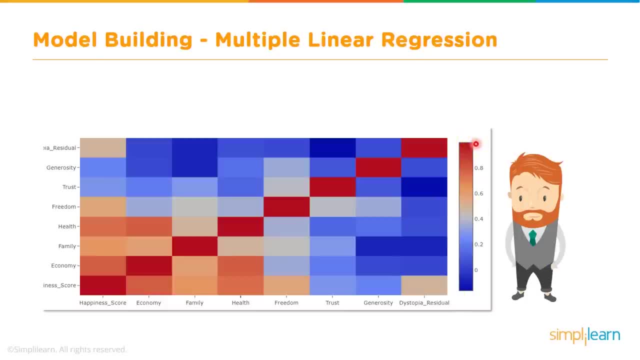 and correlation in numerical terms goes from 0 to 1, so 1 is the highest value and it can only be between 0 and 1. correlation between two variables can be only have a value between 0 and 1, so the numerical value can go from 0 to 1, and 1 here is dark color and 0 is kind of dark but it is blue. 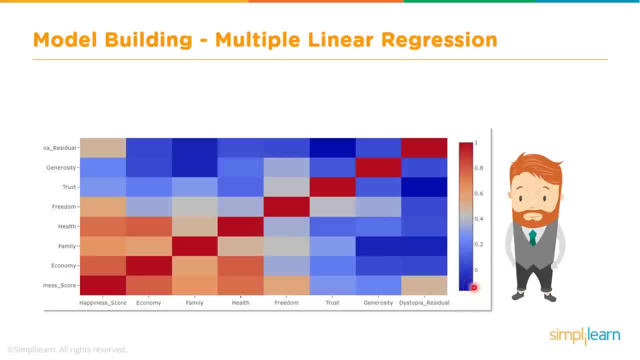 colors, from red it goes down. the dark blue color indicates pretty much no correlation. so the from this heat map we see that happiness and economy and family are probably also help, probably are the most correlated. and then it keeps decreasing after freedom, kind of keeps decreasing and coming to. 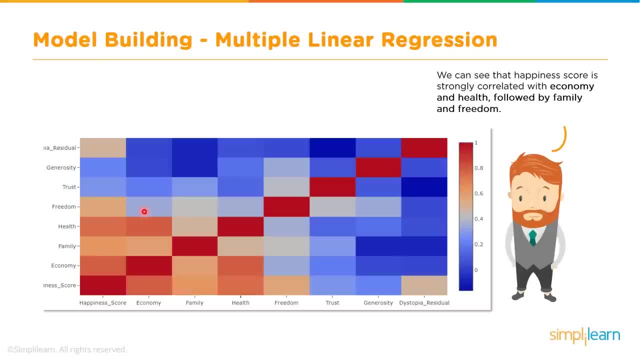 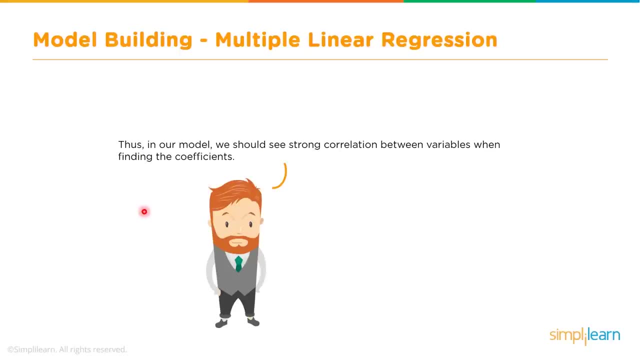 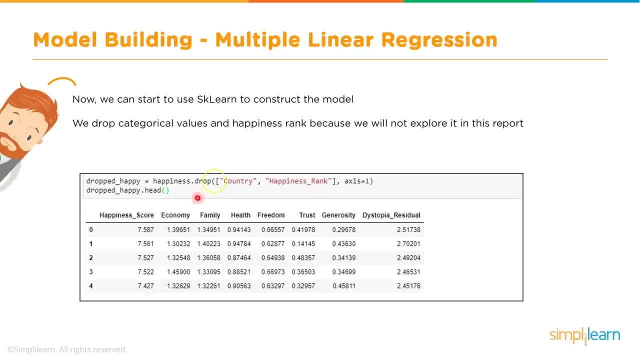 pretty much zero. all right, so that is a correlation graph, and then we can probably use this to find out which are the columns that need to be dropped, which do not have very high correlation, and we take only those columns that we will need. so this is the code for dropping some of the columns once we have prepared the data, when we 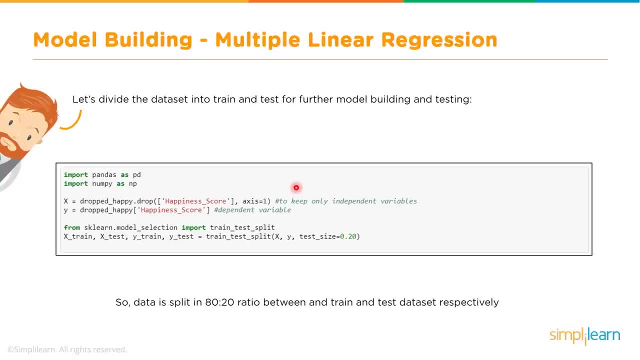 have the required columns, then we use scikit-learn to actually split the data. first of all, this is a normal machine learning process. you need to split the data into training and test data set. in this case we are splitting into 80- 20. so 80 is the training data set and 20 is the test data set. 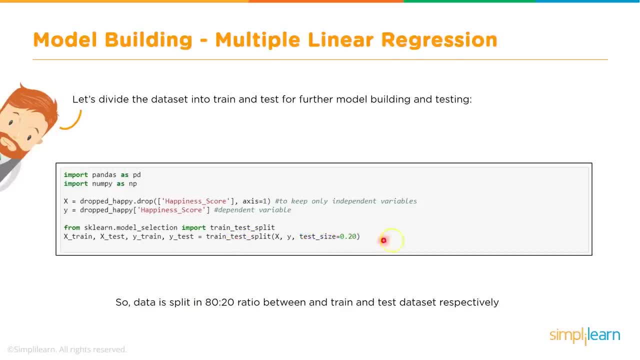 so that's what we are doing here. so we use train test split method or function. so you have all your training data, uh, in x underscore train, the labels in y underscore train. similarly, x underscore test has the test data, the inputs, whereas the labels are in y underscore test. 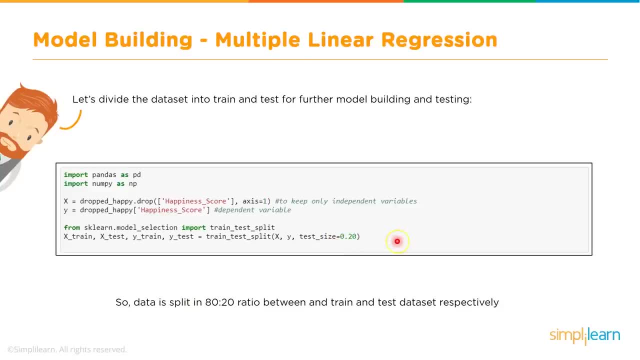 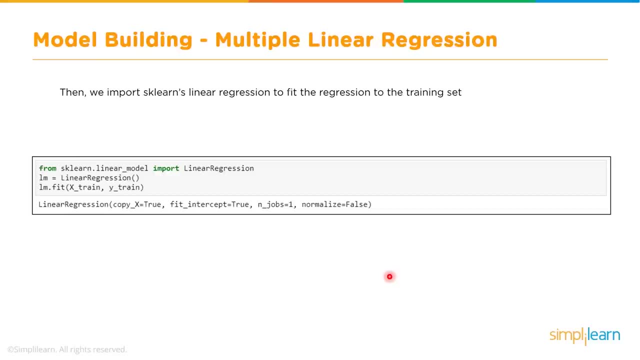 so that's all. and this value, whether it is 80, 20 or 50, 50, that is all individual preference. so in our case, we are using 80, 20.. all right, and then the next is to create a linear regression instance. so this is what we are doing: we are creating an instance of linear 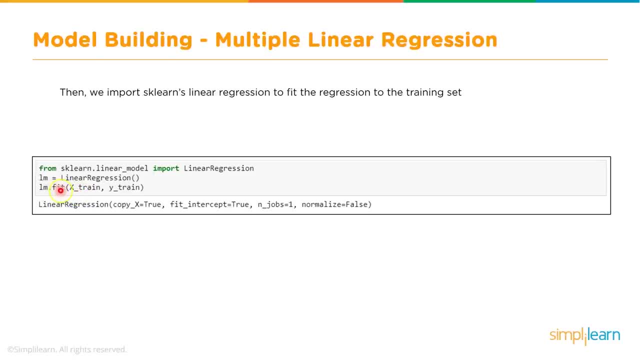 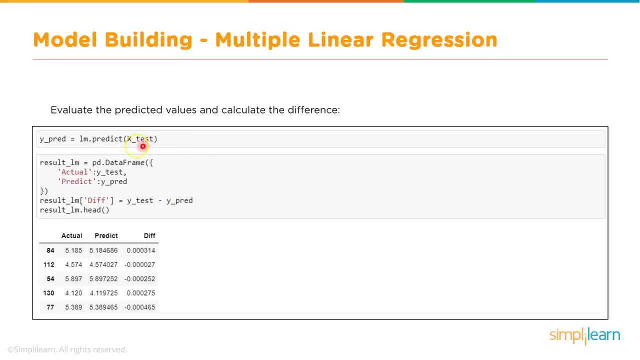 regression, and then we train the model using the fit function and we are passing x and y, which is the x value, and the label data- regular input- and the label data- label information. then we do the test, we run the or we perform the evaluation on the test data set. so this is what we are doing. 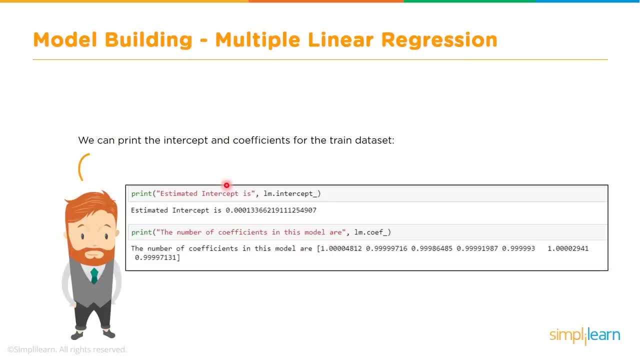 with the test data set and then we will evaluate how accurate the model is and using the scikit-learn functionality itself, we can also see what are the various parameters and what are the various coefficients, because in linear regression you will get like a equation of, like a straight line: y is equal to beta 0 plus beta 1 x 1 plus beta 2 x 2, so those beta 1 beta. 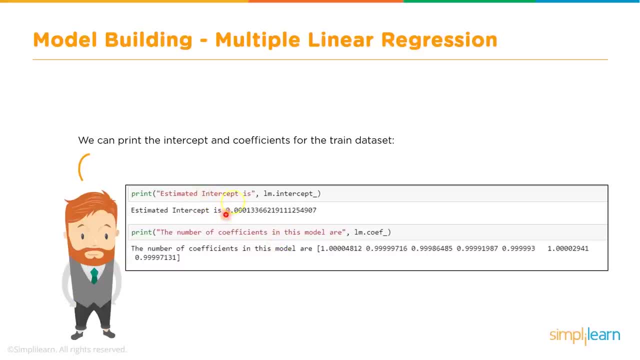 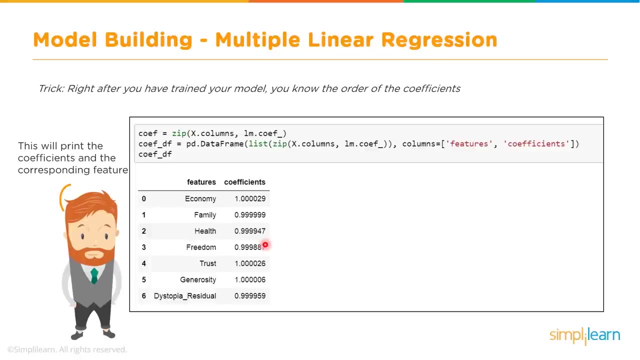 2, beta 3 are known as the coefficients and beta 0 is the intercept. after the training, you can actually get these information of the model- what is the intercept value, what are the coefficients, and so on- by using these functions. so let's take quickly, go into the lab and 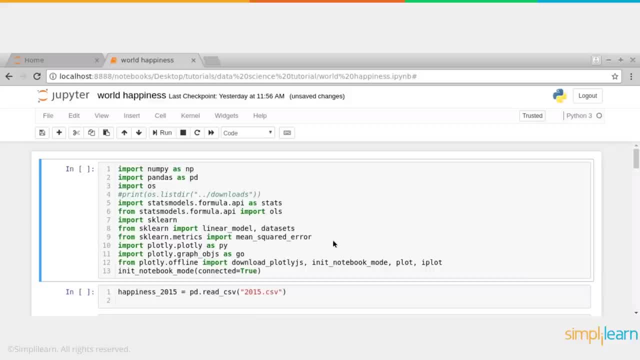 take a look at our code. okay, so this is my lab, this is my jupyter notebook where the code. i have the actual code and i will take you through this code to run this linear regression on the world happiness data. so we will import a bunch of libraries, numpy, pandas, plot plotly and so on. 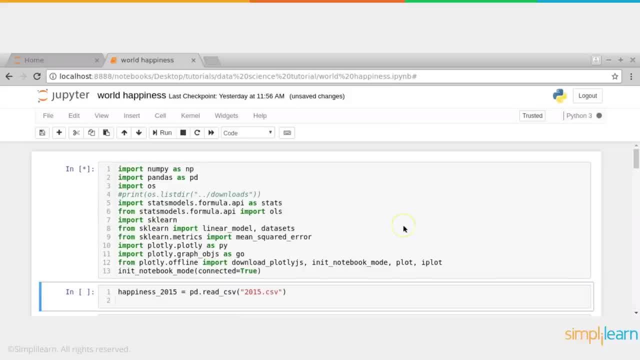 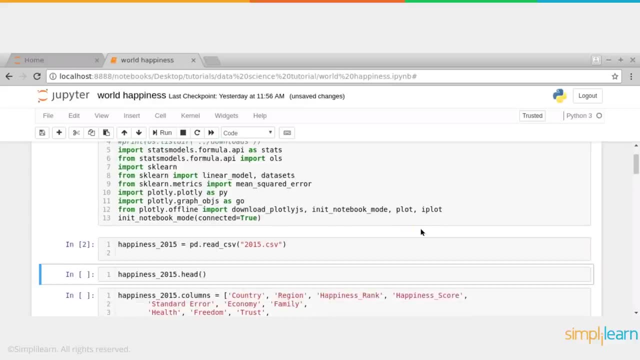 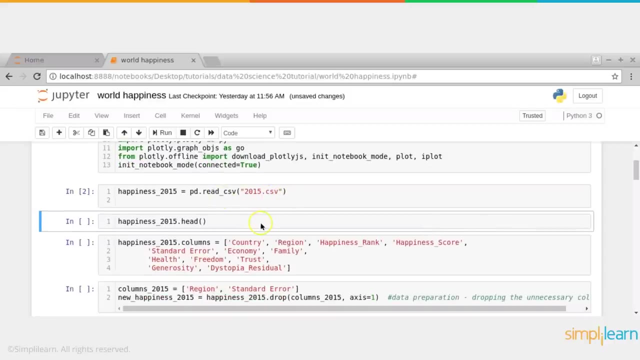 also, yeah, scikit-learn. that's also very important. so that's the first step. then i will import my data, and the data is in three parts. there are three files, one for each year- 2015, 2016 and 2017- and it is a csv file. so i've imported my data. let's take a look at the data. 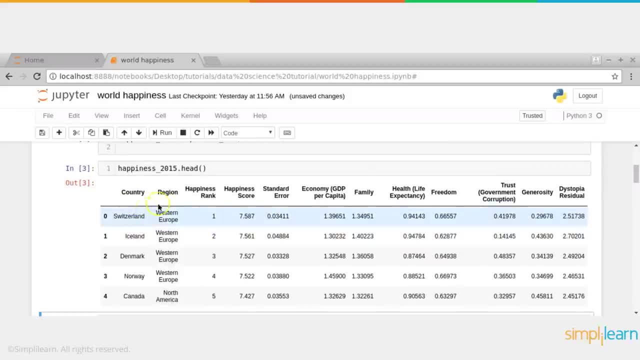 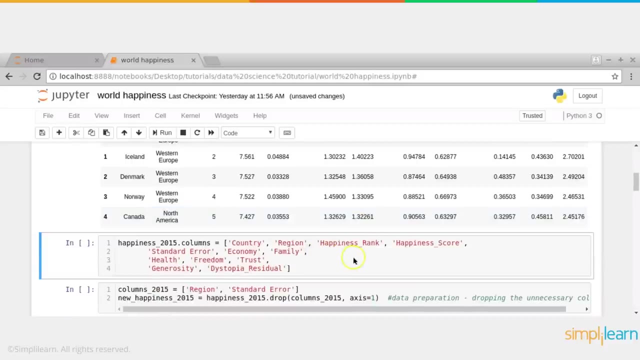 quickly glance at data. so this is how it looks. we have the country, region, happiness rank and then happiness score, there are some standard errors, and then what is the per capita family, and so on. so, and then we will keep going. we will create a list of all these column names we will be using later. so for now, just i will run this code and no need of. 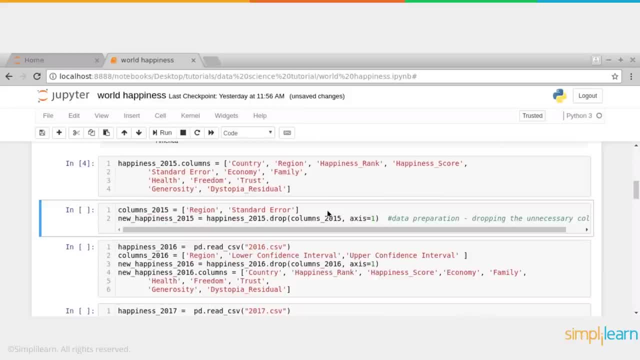 major explanation. at this point. we know that some of these columns probably are not required, so you can use this drop functionality to remove some of the columns which we don't need, like, for example, region and standard. error will not be contributing to our model, so we will basically drop those. 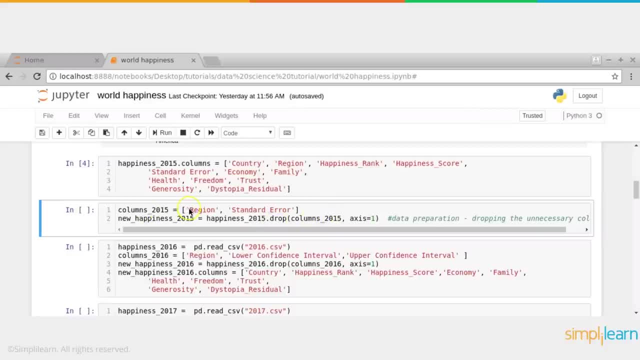 values out here. so we use the drop and then we created a vector of it. these names column names. that's what we are passing here. instead of giving the names of the columns here, we can pass a vector, so that's what we are doing. so this will drop from our data frame. it will. 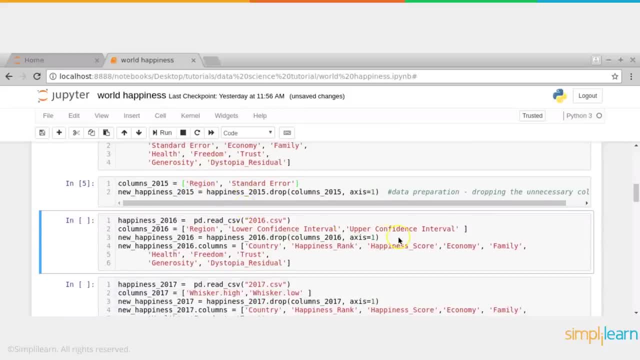 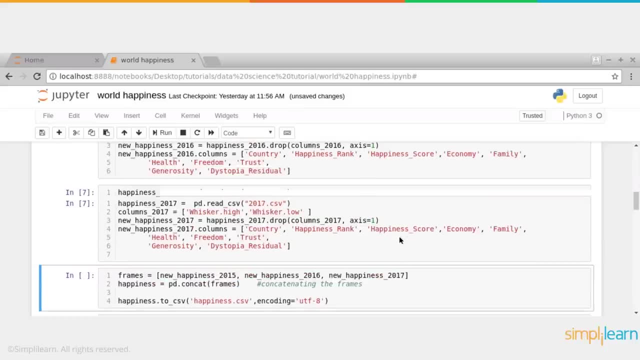 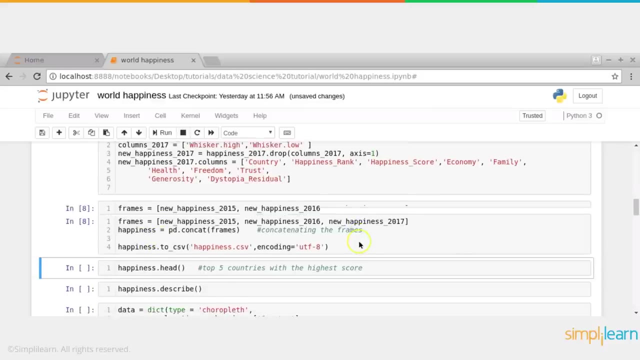 remove region and standard error, these two columns. then the next step: we will read the data for 2016 and also 2017, and then we will concatenate this data. so let's do that. so we have now data frame called happiness, which is a concatenation of both- all the three files. 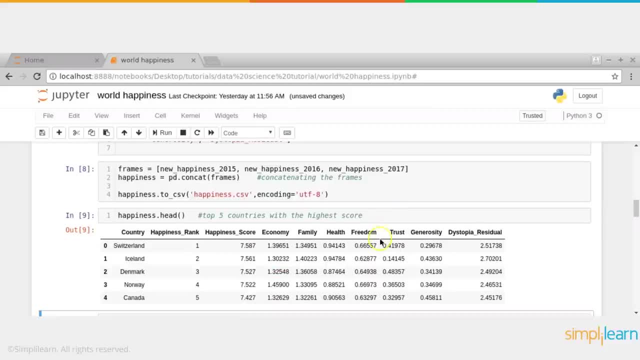 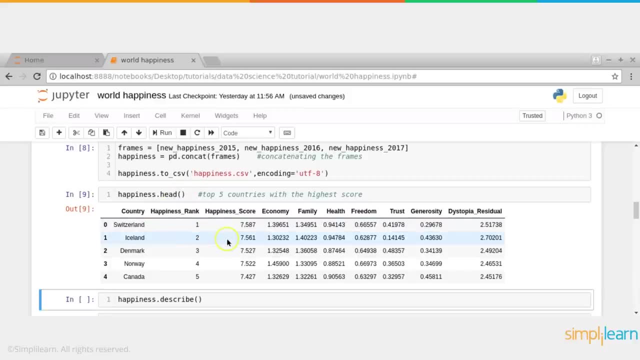 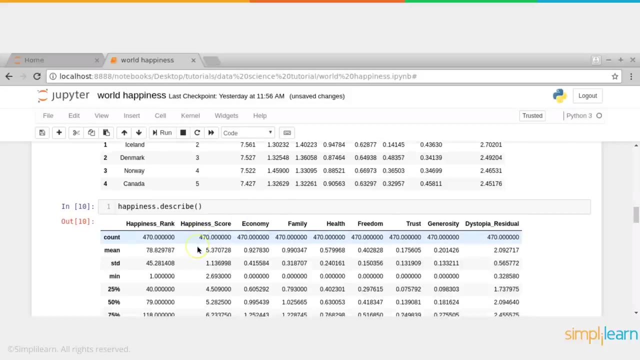 let's take a quick look at the data now. so most of the unwanted columns have been removed and you have all the data in one place for all the three years, and this is how the data looks. and if you want to take a look at the summary of the columns, you can say describe and you will get this. 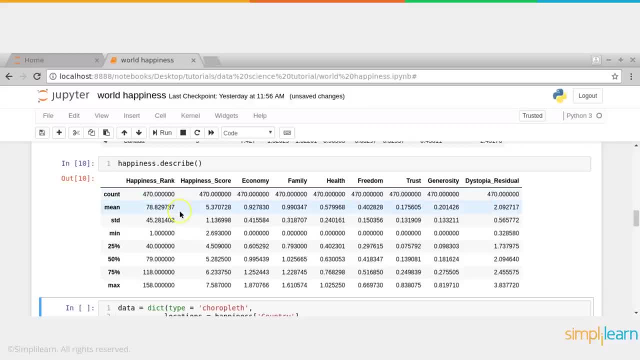 information, for example, for each of the columns: what is the count, what's, what is the mean value? standard deviation, especially the numeric values, okay, not the categorical values. so this is a quick data is and initial little bit of exploratory analysis can be done here. so what is the maximum? 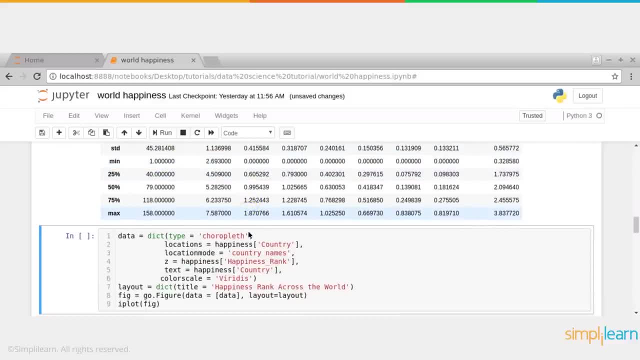 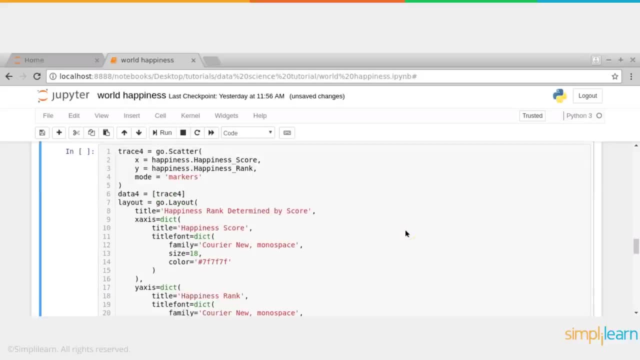 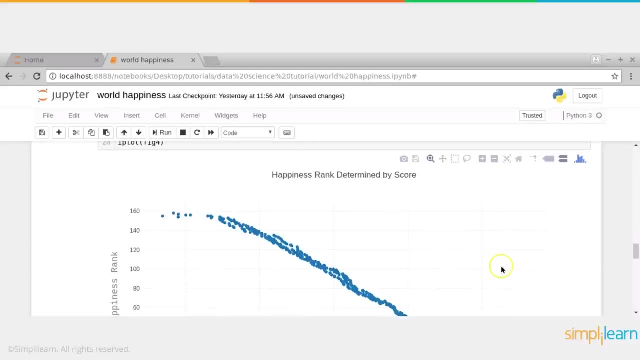 value, what's the minimum value, and so on for each of the columns. all right, so then we go ahead and create some visualizations using plotly. so let us go and build a plot. so if we see here now, this is the relation correlation between happiness rank and happiness score, this is what we have seen. 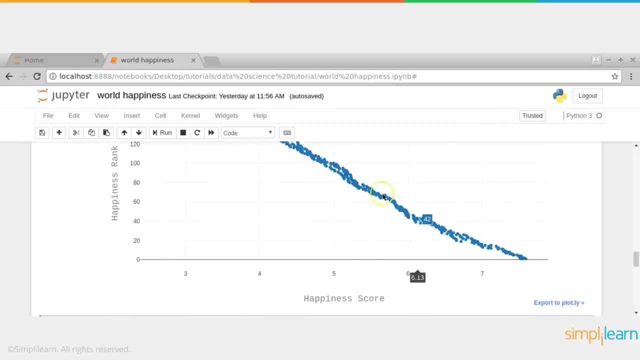 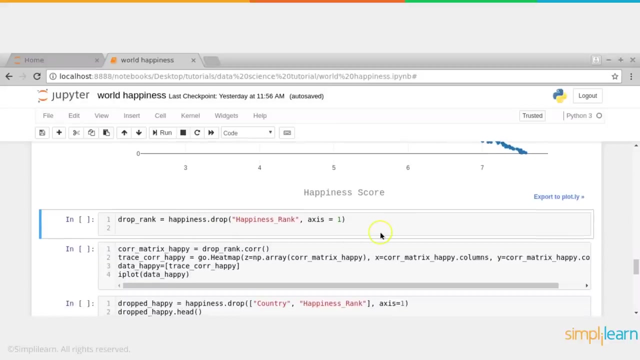 in the slides as well, we can see that there is a correlation between them. only thing is it is inverse correlation, but otherwise they are very tightly correlated, which also says that they both probably provide the same information. so there is no, not much of value add, so we'll go ahead and drop the happiness rank as well. 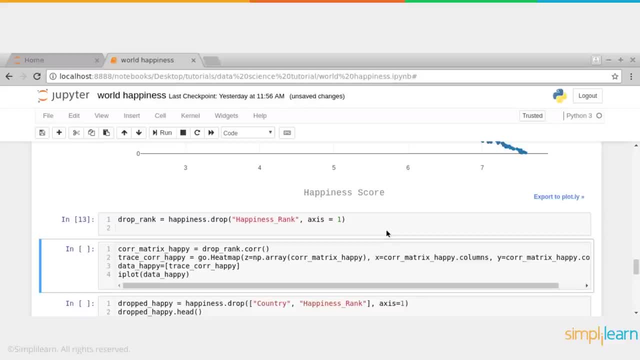 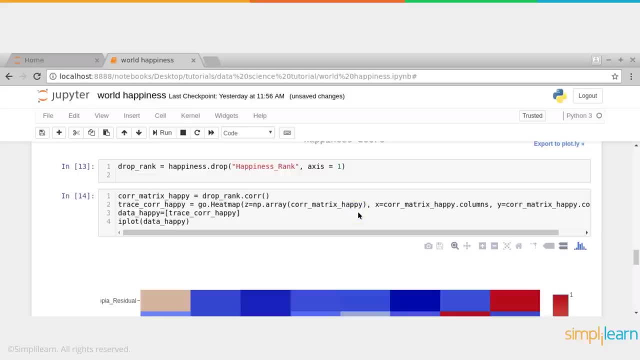 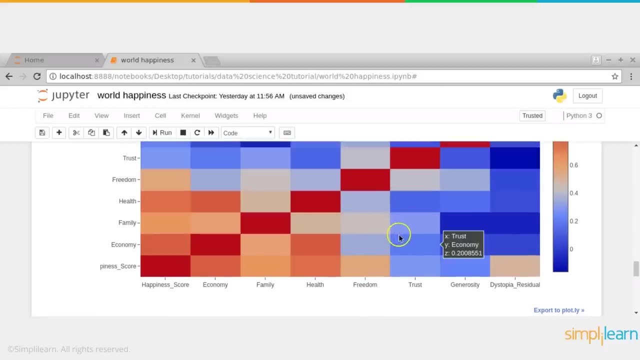 from our columns. so that's what we're doing here and now we can do the creation of the correlation heat map. let us plot the correlation heat map to see how each of these columns is going to be correlated to the others, and we, as we have seen in the slides, this is how it looks. so 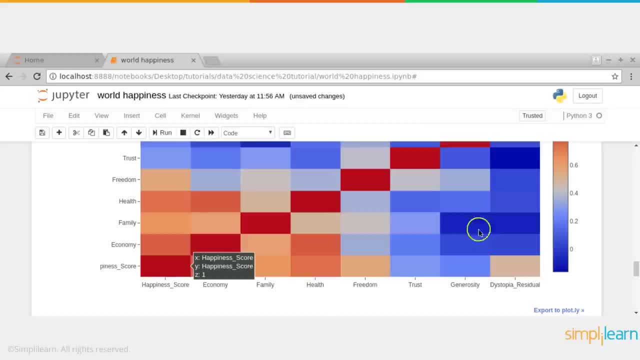 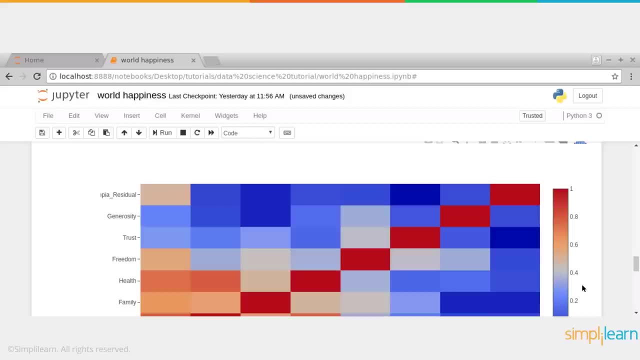 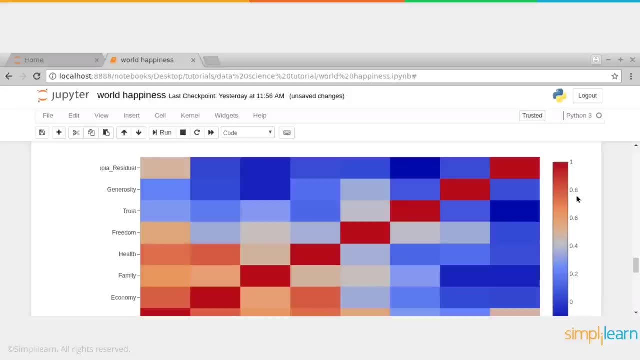 happiness score is very highly correlated. so this is the legend we have seen in the slide as well. so blue color indicates pretty much zero or very low correlation. deep red color indicates very high correlation and the value correlation is a numeric value and the value goes from 0 to 1.. 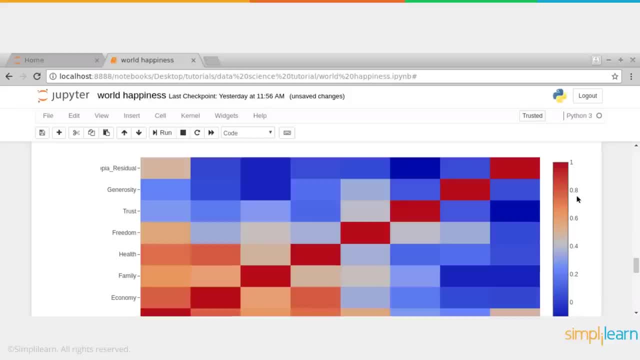 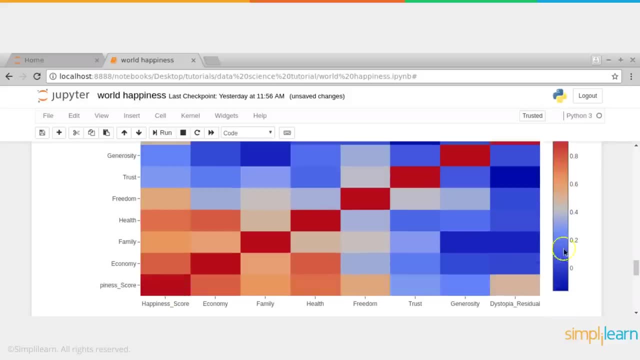 if the two items or two features or columns are highly correlated, then they will be as close to 1 as possible, and two columns that are not at all correlated will be as close to zero as possible. so that's how it is, for example, here, happiness score and happiness score every column or every. 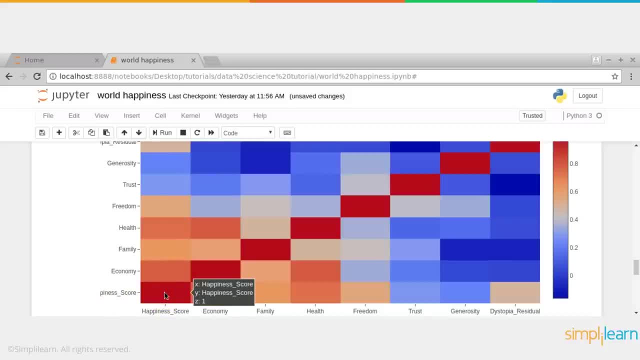 feature will be highly correlated to itself. so it is like between them there will be correlation, value will be one, so that's why we see deep red color, but then others are. for example, with higher values are economy and then health, and then maybe family and freedom. so these are generosity and 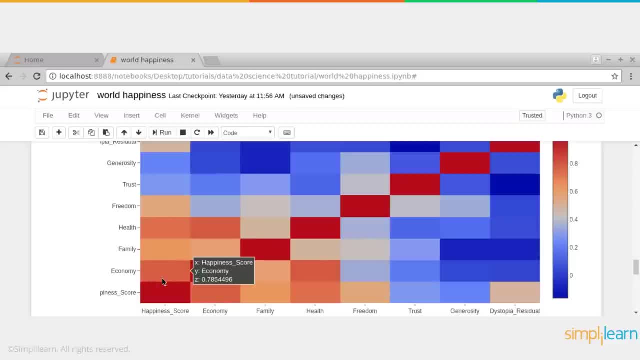 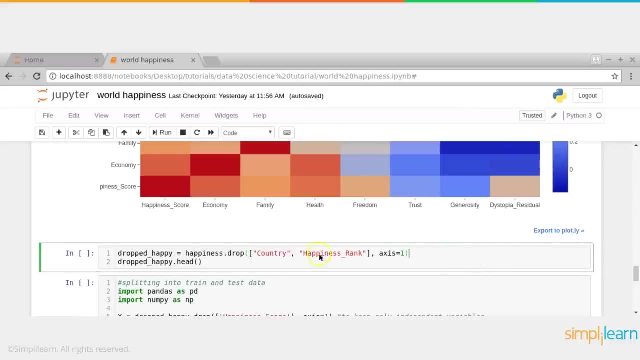 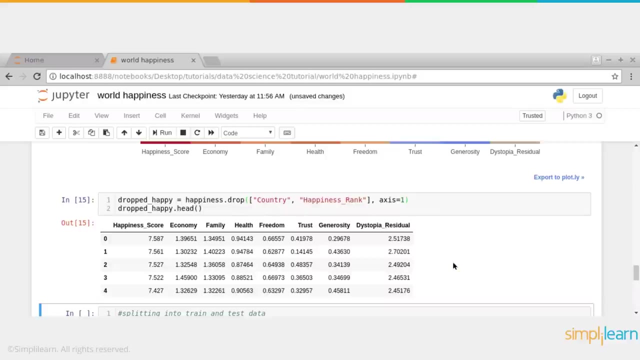 trust are not very highly correlated to happiness score. so that is, uh, one quick exploratory analysis we can do and therefore we can drop the country and the happiness rank, because they also, again, don't have any major impact on the analysis, on our analysis. so now we have prepared our data, there was no need to clean the data, because the data 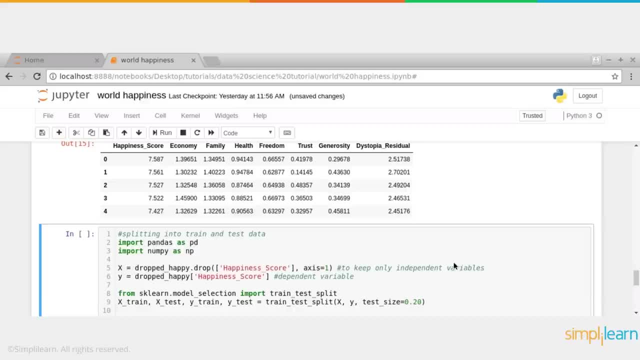 was clean, but if there were some missing values and so on, as we have discussed in the slides, we would have had to perform some of the data cleaning activities as well. but in this case the data was clean. all we need to do is clean the data and then we can drop the country and the happiness score. 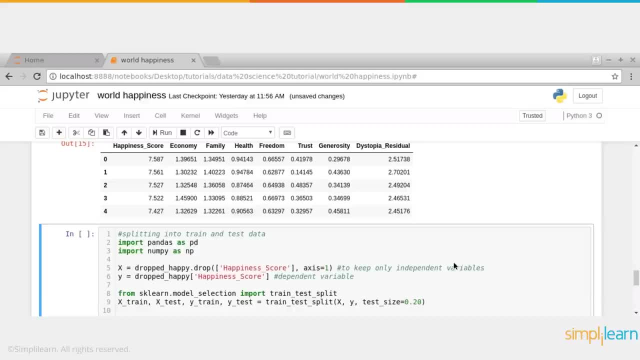 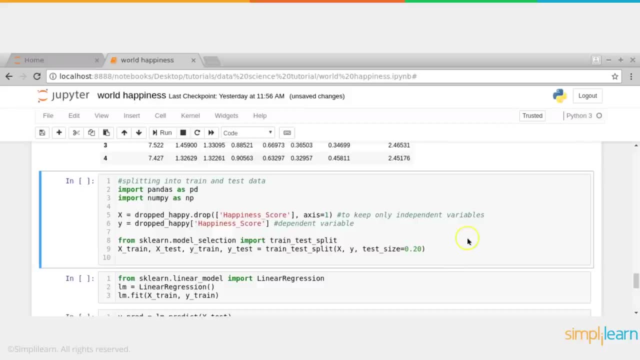 needed to do was just the preparation part. so we removed some unwanted columns and we did some exploratory data analysis. now we are ready to perform the machine learning activity. so we use scikit-learn for doing the machine learning. scikit-learn is python library that is available. 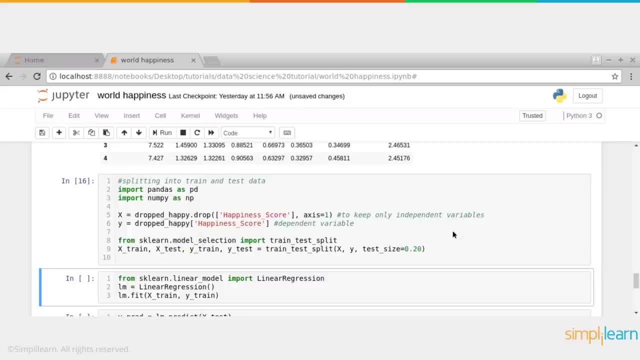 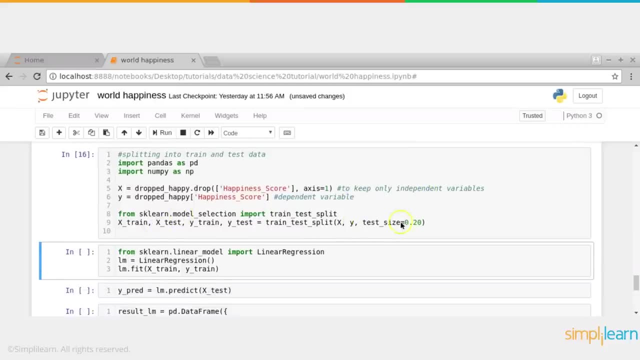 for performing our machine learning. once again, we will import some of these libraries, like pandas and numpy and also scikit-learn. first step we will do is split the data in 2080 format so you have all the test data, which is 20 of the data is test data and 80 is your. 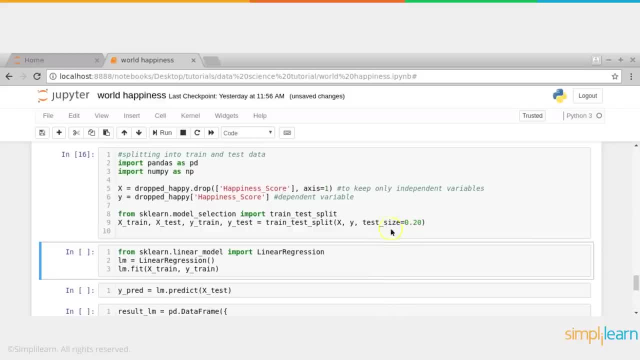 training data. so this test size indicates how much of it is the. what is the size of the test data? so remaining, which is? uh, here we are saying 0.2. therefore, that means training is 0.8, so training data is 80 percent. all right, so we have executed that, split the data and now we create an instance. 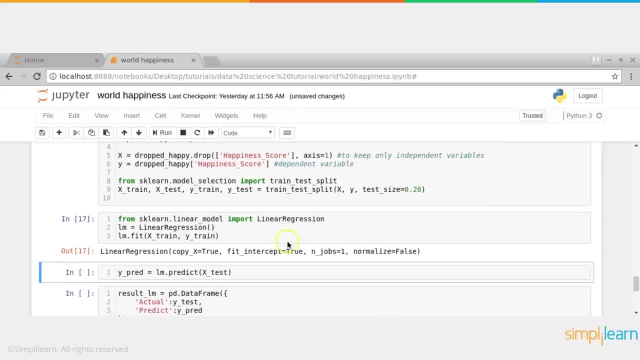 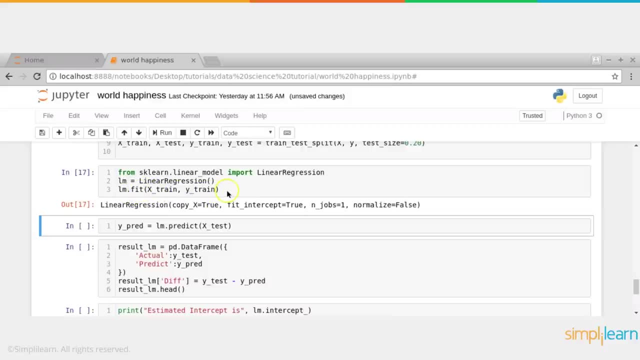 of the linear regression model. so lm is our linear regression model and we pass x and y, the training data set, and call the function fit so that the model gets trained. so now, once that is done, training is done, training is completed. and now what we have to do is we need to predict. 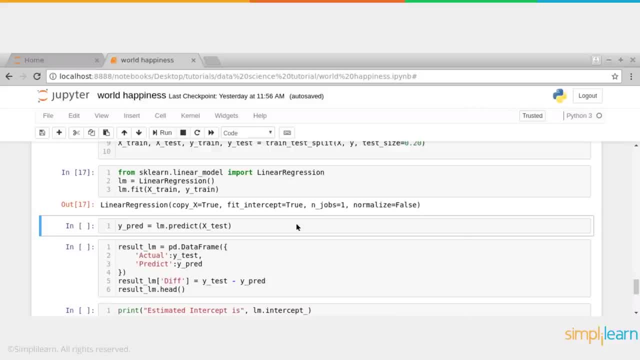 the values for the test data. so the next step is using. so you see a fit will basically run the training method. predict will actually predict the values. so we are passing the input values, which is the independent variables, and we are asking for the values of the dependent. 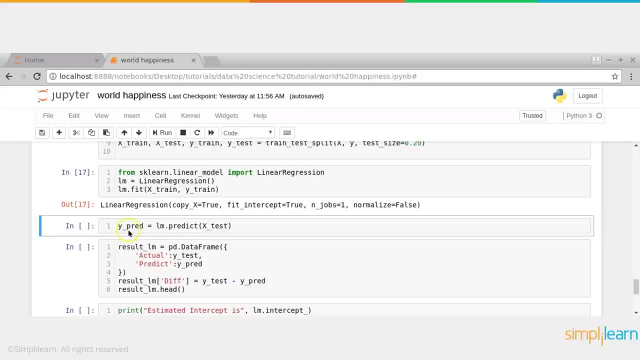 variable, which is which we are capturing in y underscore track, and we use the predict method here. lm dot predict, so this will give us all the predicted y values and remember we already have y underscore test- has the actual values, which are the labels, so that we can use these two to compare. 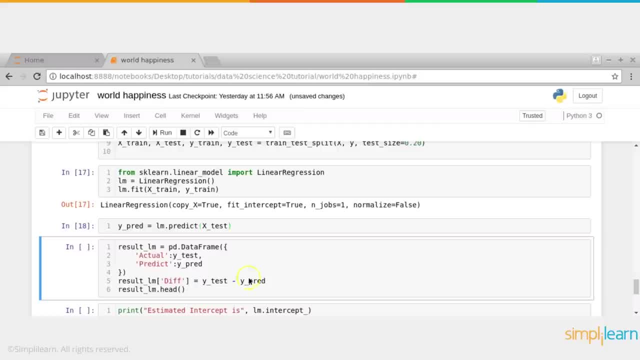 and find out how much of it is error. so that's what we are doing here: we are trying to find the difference between the predicted value and the actual value. y underscore test is the actual value for the test data and y underscore predict is the predicted value. we just found out the predicted value, so 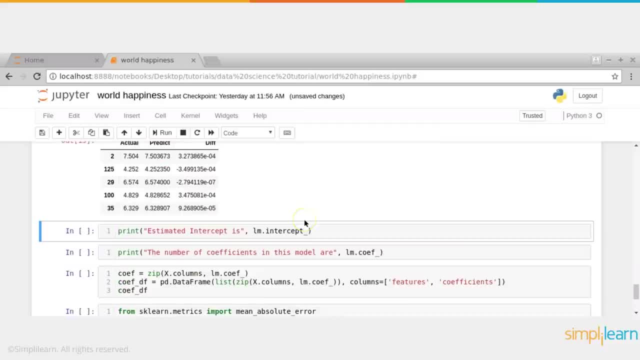 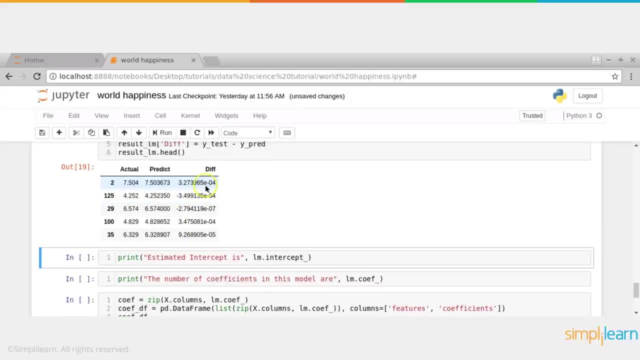 we will run that and we can do a quick check as to how the data looks. how is the difference? so? in some cases it is positive, some cases it is negative, but in most of the cases i think the difference is very small. this is exponential to the power of 0 minus 0, 4 and so on. so looks like. 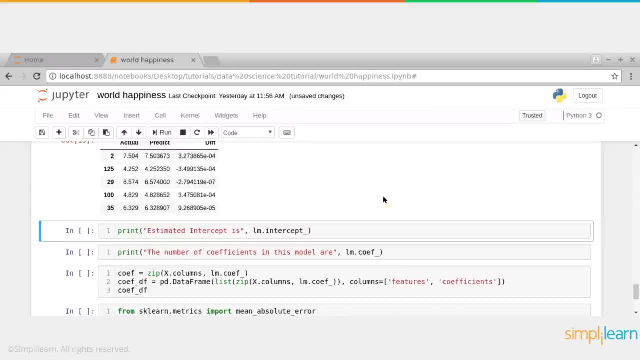 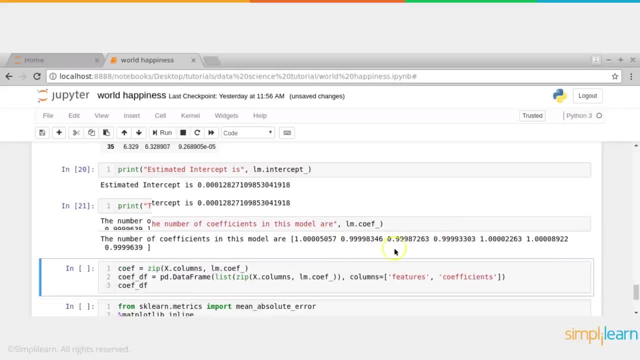 our model has performed reasonably well. we can now check some of the parameters of our model, like the intercept and the coefficients. so that's what we are doing here. so these are the coefficients of the various parameters, that we are the coefficients of the various independent variables. okay, so these are the 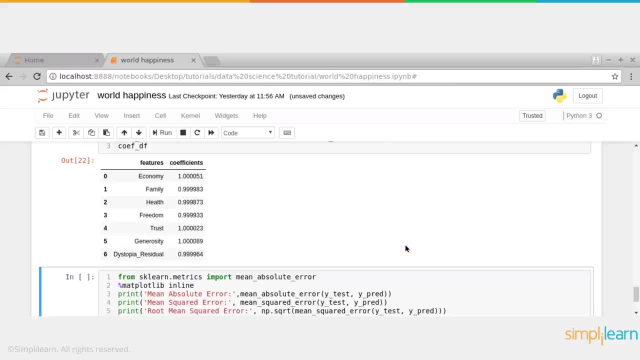 values. then we can quickly go ahead and list them down as well, against the corresponding independent variable. so the coefficients against the corresponding independent variable. so one point zero, zero, five, one is the coefficient for economy. point nine, nine, nine, eight, three is for family: coefficient for family and health, and so on and so forth. right, so that's what this is, uh. 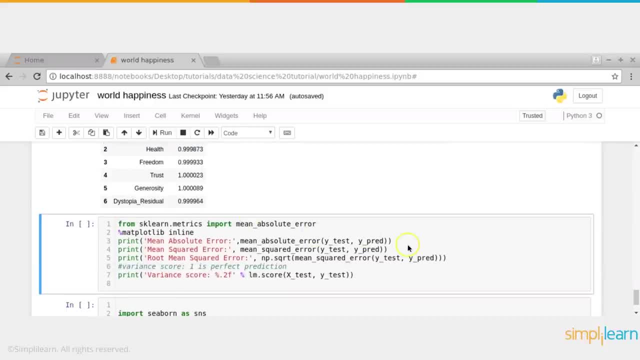 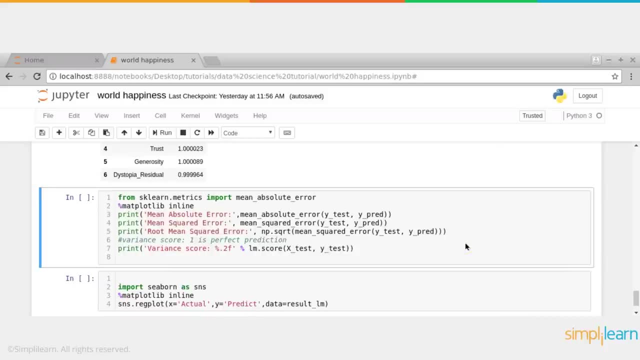 showing. now we can use the functionality- readily available functionality- of scikit-learn and then plot that to find some of the parameters which determine the accuracy of this model, like, for example, what is the mean square error, and so on. so that's what we are doing here, so let's just go. 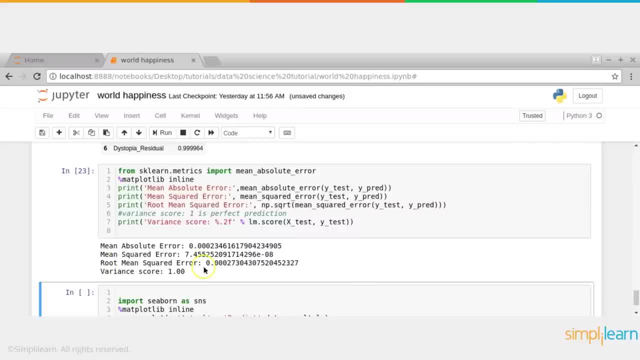 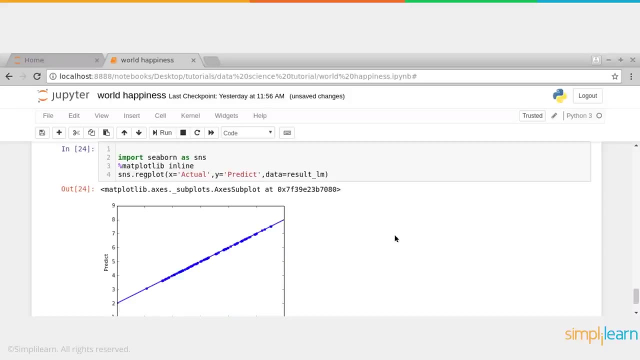 ahead and run this, so you can see here that the root mean square error is pretty low, which is a good sign and which is a one of the measures of how well our model is performing. we can do one more quick plot to just see how the actual values and the predicted values are looking, and once 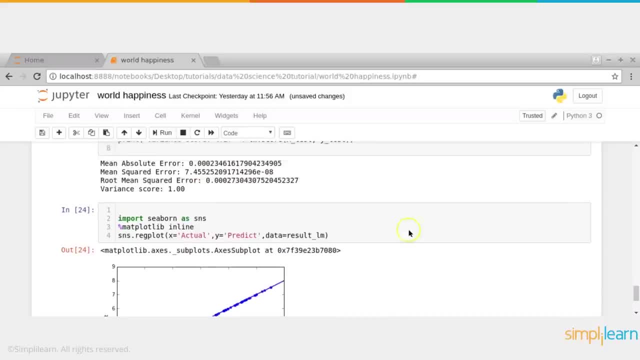 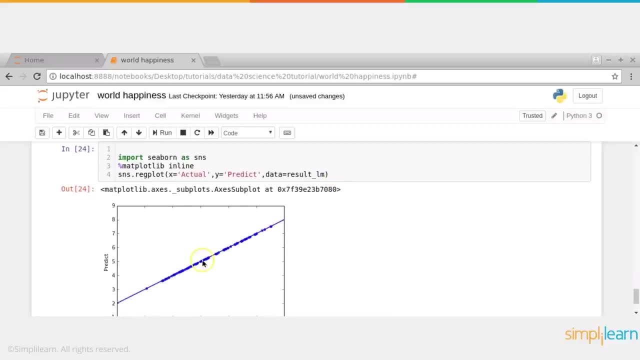 again, you can see that, as we have seen from the root mean square error, root mean square error is very, very low. that means that the actual values and the predicted values are pretty much matching up, almost matching up, and this plot also shows the same. so this line is going through the predicted. 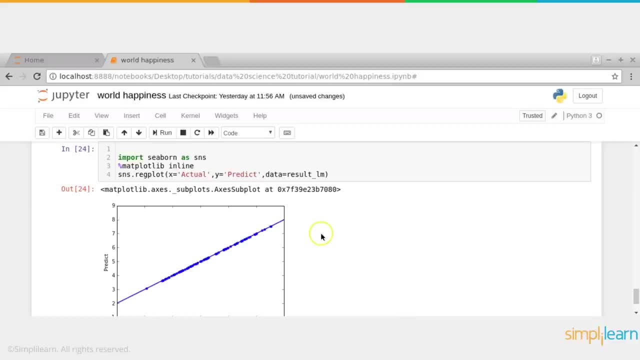 values and the actual values, and the difference is very, very low. so again, this is actually data. this is one example where the accuracy is high and the predicted values are pretty much matching with the actual values. but in real life you may find that these values are slightly more scattered and you may get the error. value can be relatively. 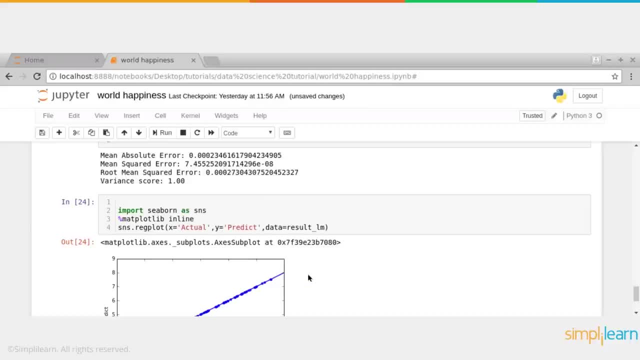 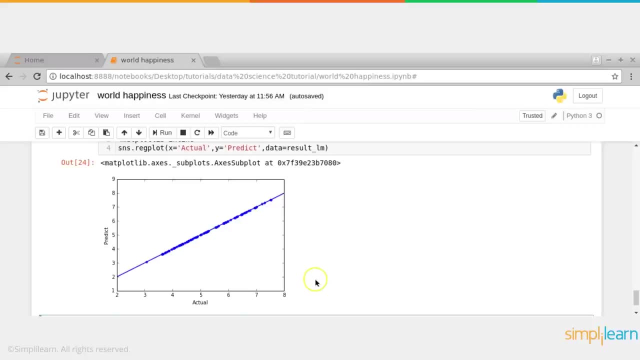 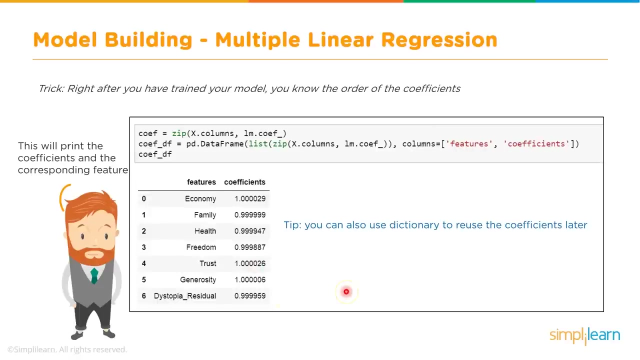 on the higher side, the root mean square. okay, so this was a good, quick example of the code to perform data science activity or a machine learning or data mining activity. in this case, we did what is known as linear regression. so let's go back to our slides and see what else is. 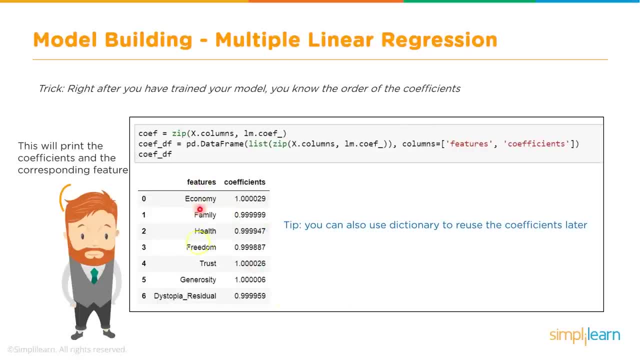 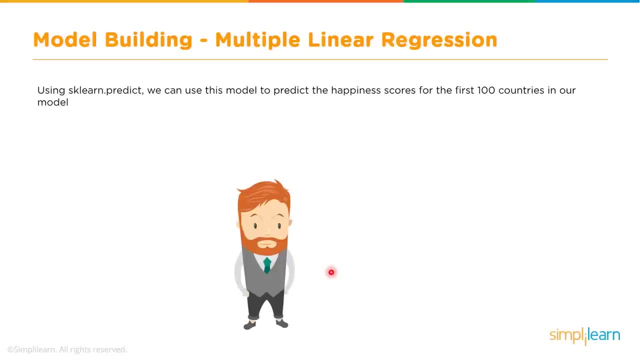 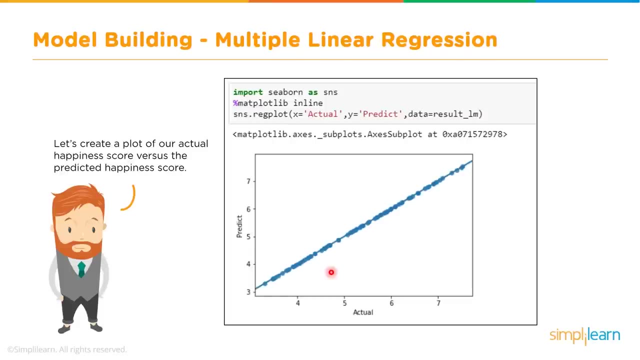 there. so we saw this. these are the coefficients of each of the features in our code, and we have seen the root mean square error as well, and with we can take a few hundred countries, certain values and actually predict to see if how the model is performing, and I think we have done this as well. 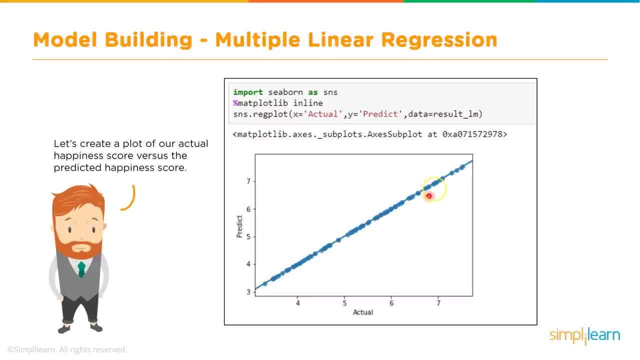 and in this case, as we have seen, the pretty much the predicted values and the actual values are pretty much matching, which means our model is almost 100 accurate, as I mentioned it. real life it may not be the case, but in this particular case we have got a pretty good model which is: 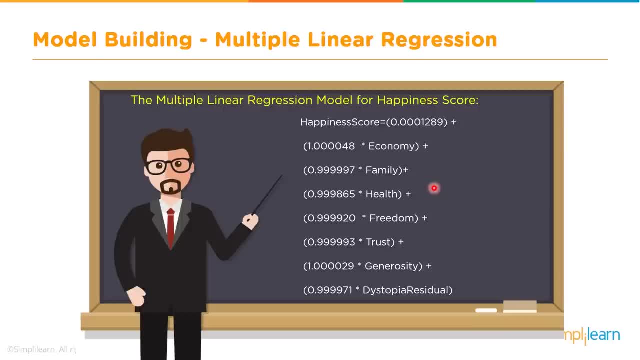 very good. also, subsequently, we can assume that this is how the equation in linear regression- the model is nothing but an equation like y- is equal to beta 0 plus beta 1 x 1 plus beta 2 x 2 plus beta 3 x 3, and so on. so this is what we are showing here, so this is our intercept, which. 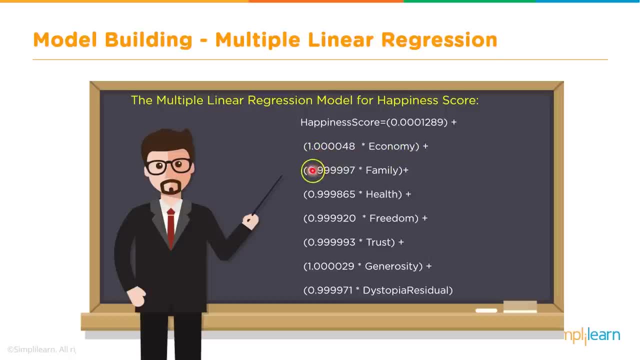 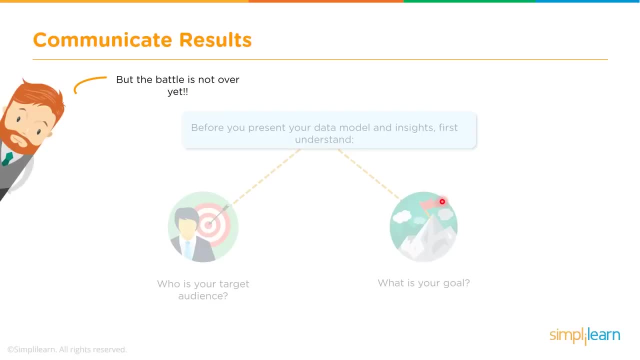 is beta 0, and then we have beta 1 into economy value, beta 2 into the family value, beta 3 and 3 into health value, and so on. so that is what is shown here, okay, so I think the next step, once we have the results from the data mining or machine learning activity, the next step is to communicate. 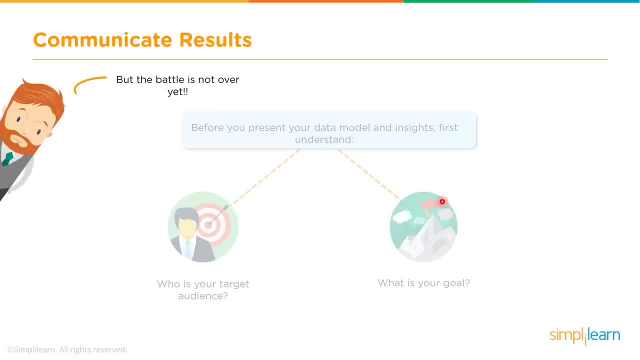 these results to the appropriate stakeholders. so that is what we will see here now. so how do we communicate? usually, you take these results and then either prepare a presentation or put it in a document and then show them these actionable results or actionable insights, and you need to find out who are your target audience and put all the results in context. 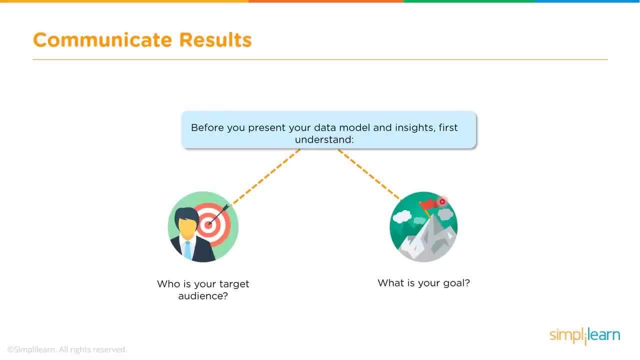 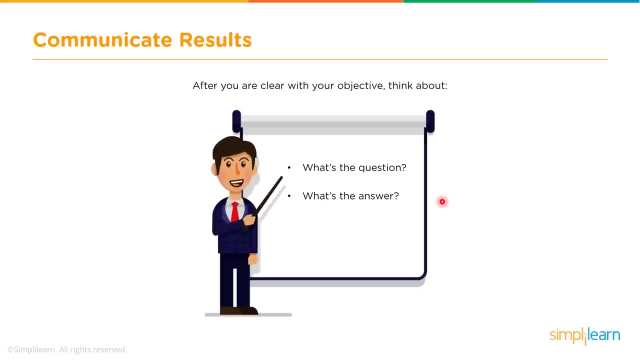 and maybe if there was a problem statement, you need to put this results in the context of the problem statement. what was our initial goal that we wanted to achieve so that we need to communicate here based on? I remember we started off with what is the question and what is the data. 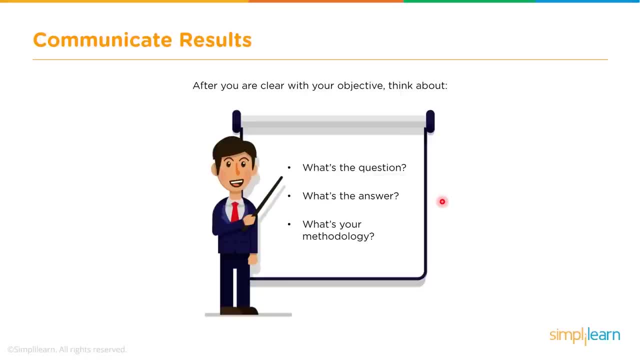 and so on. and then what is the answer? so we we need to put the results. and then What is the methodology that we have used? All that has to be put and clearly communicated in business terms so that the people understand very well from a business perspective. 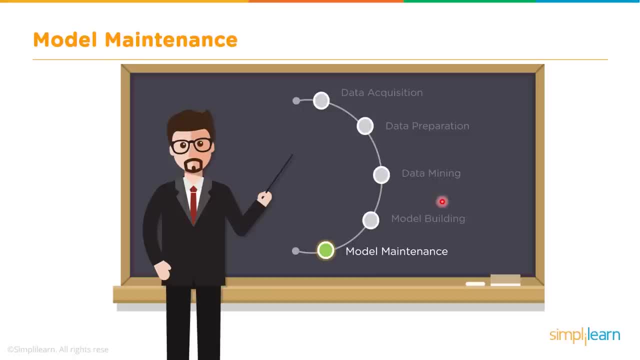 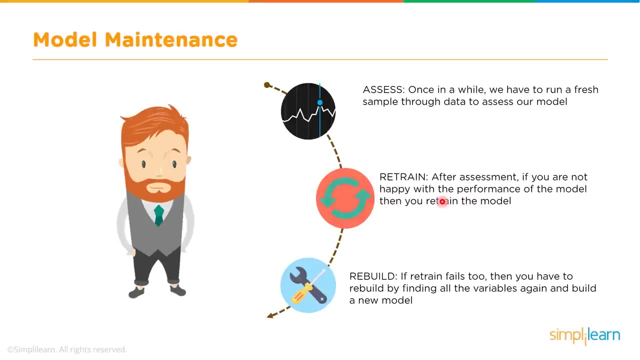 So, once the model building is done, once the results are published and communicated, the last part is maintenance of this model. Now, very often, what can happen is the model may have to be subsequently updated or modified because of multiple reasons. Either the data has changed. 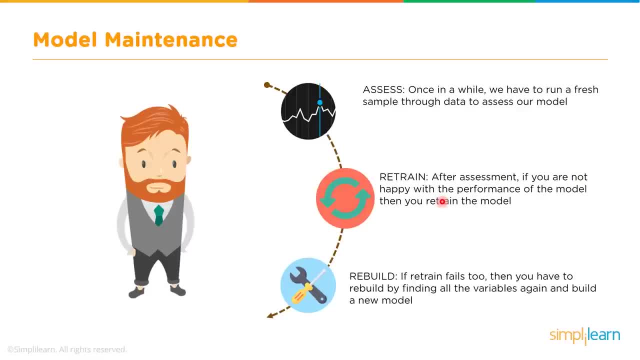 the way the data comes has changed, or the process has changed, or for whatever reason. the accuracy may keep changing. Once you have trained the model, for example, we got a very high accuracy, but then, over a period of time, there can be various factors which can cause that. 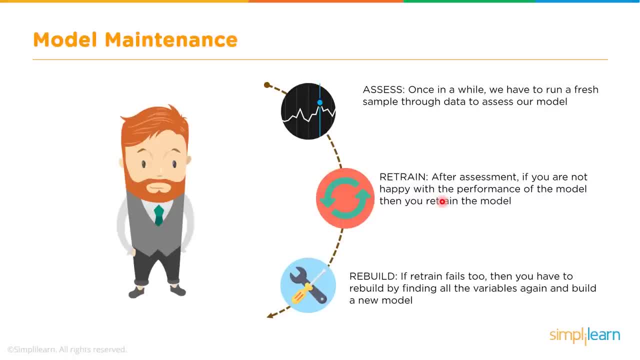 So from time to time we need to check whether the model is performing well or not. The accuracy needs to be tested once in a while And, if required, you may have to rebuild or retrain the model. So you do the assessment. 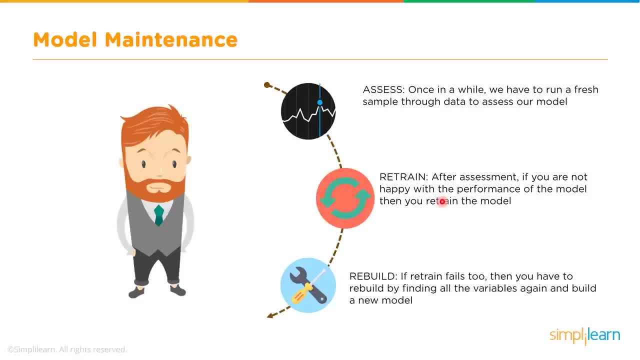 you see if it needs any tweaks or changes and then, if it is required, you need to probably retrain the model with the latest data that you have and then you deploy it. You build the model, train it and then you deploy it. 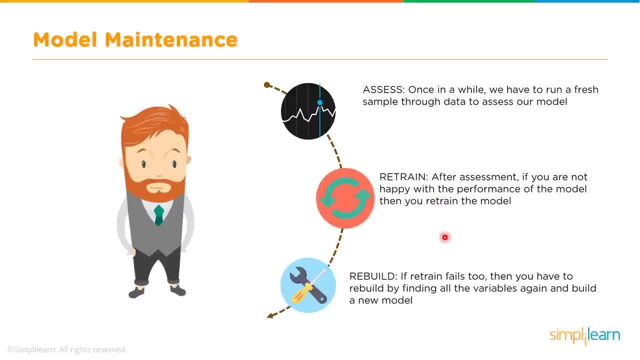 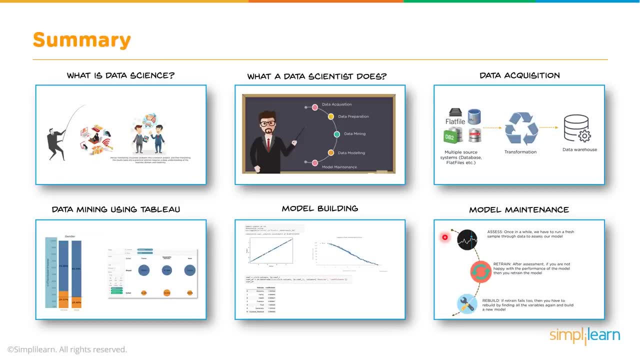 So that is like the maintenance cycle that you may have to take the model through. All right, so we are pretty much at the end of our tutorial. So what did we learn in this tutorial? We talked about what is data science and who is a data scientist. 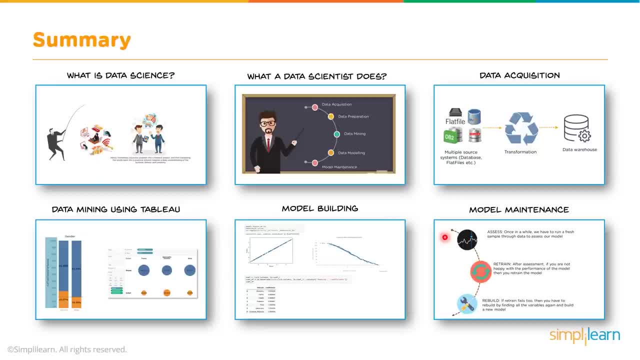 Then we talked about what a data scientist performs or does a day in the life of a data scientist. Some of the activities or the methodologies, like the processes, data acquisition, data preparation, mining and model building, and so on, And then, last but not least, the model maintenance. 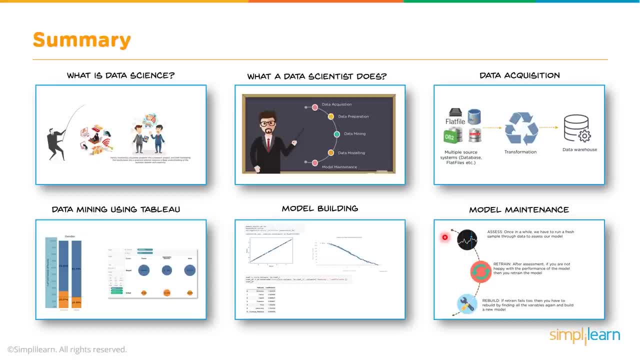 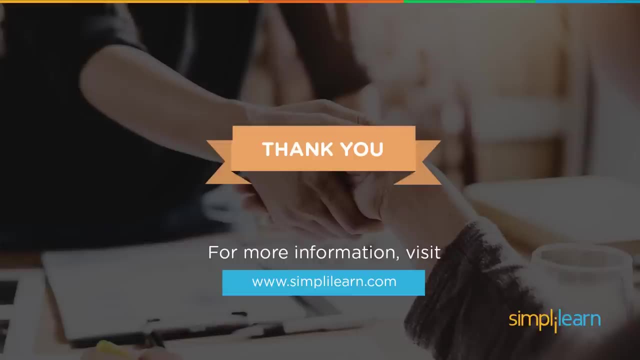 And in the process we have also taken a look at the Python code that was used for performing a linear regression model: creating a linear regression model, training it and testing it and checking the various parameters of that model. With that, we come to the end of this tutorial.